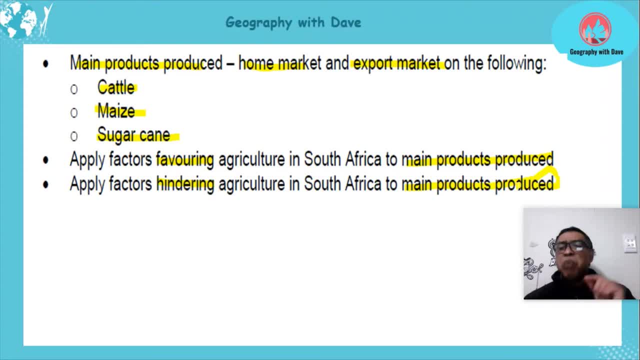 products produced. i will also look at the importance of the product itself. now, in many occasions, regarding factors favoring, hindering and the importance, you may find that the factors are similar as we move through the lesson. okay, so my apologies for using up your data, that i may repeat things, but the difference is i will use different examples which are specific. 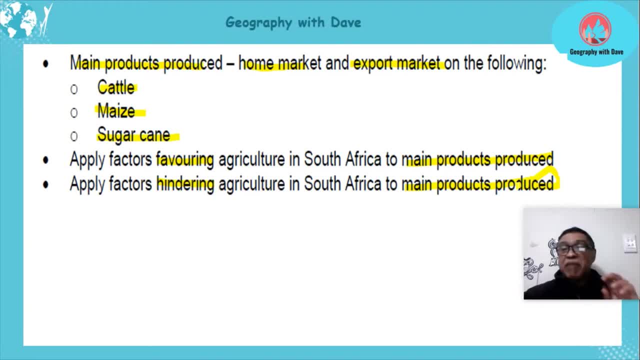 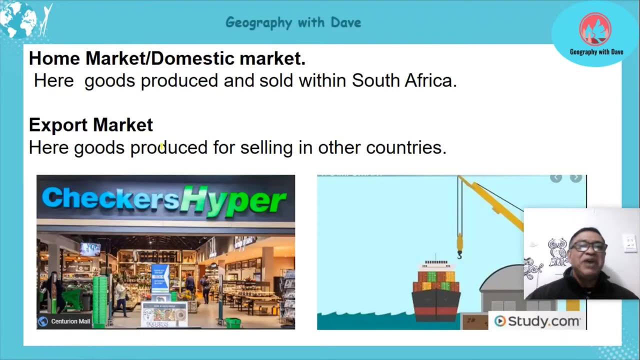 to either beef maize or uh, or cattle maize or sugarcane, and that is why i'll go over them each time. so my apologies again for data usage, but it's necessary. okay, learners, let's go further, right, obviously, if we're going to link it to the home and export. 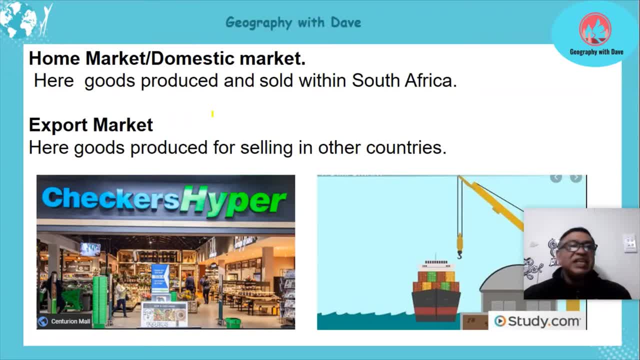 market. we need to have an understanding of what's the home market and what's the export market- very important for us. okay, now let's look at what's the home market also called in many texts, you'll see it: it's called the domestic market. domestic means local. 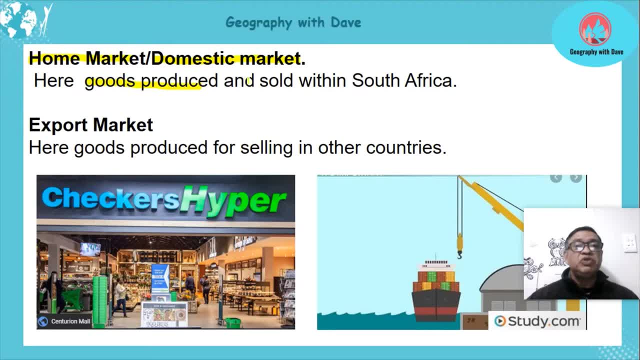 okay, so, yeah, goods are produced. well, obviously, it's always produced in south africa, whether it's home and export market, and it's the main words. it's sold within south africa. all right, yeah, the goods are sold within south africa, okay, okay, now export market, and it comes from the term export, because we are selling. 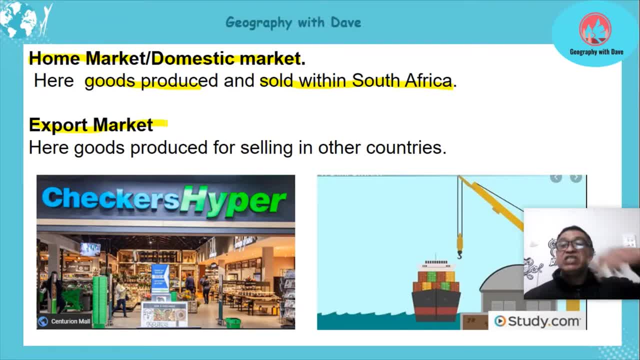 exporting means selling it to or sending it to other countries, and it comes from that explanation itself. here goods are produced for selling to other countries. all right, so our hypermarket here. of course it may consist of goods from from overseas, but lots of the goods are found here, are produced in the country for the people of South Africa. okay, checkers here. 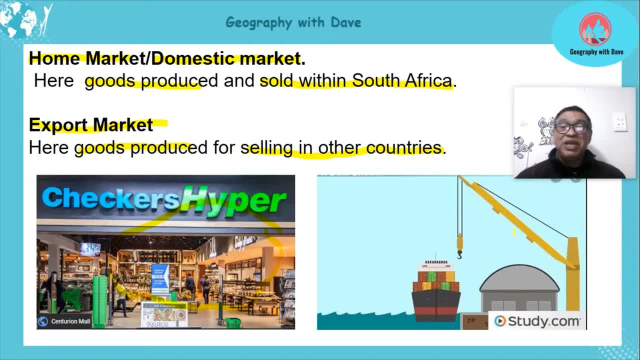 I'm going to take the sketch as if we have loaded the ship, okay, and it's going out of the harbor to another country, all right. so that's exporting, so we produce the goods and we sent it away. it's nice to have a visual of it. all right, so we've got an understanding of that, because we're 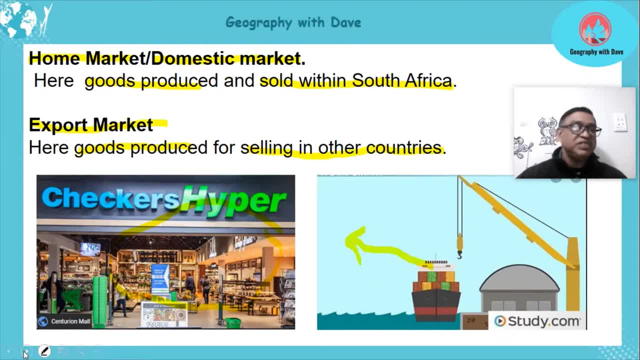 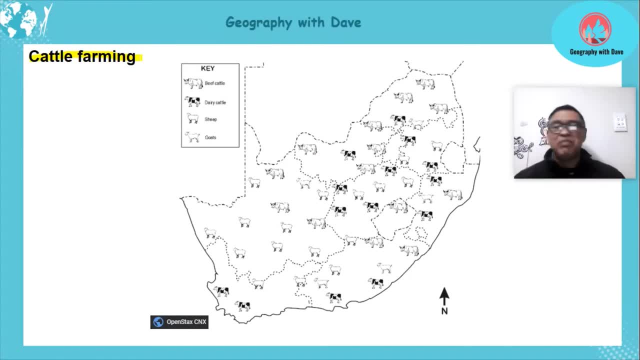 going to apply it in our explanations. all right, now we're going to start off with cattle farming, cattle farming itself, and if you look at this, my apologies, I'm a bit thirsty today. what, if you look at this? each symbol here, okay, cattle, that's beef cattle, dairy cattle, and then 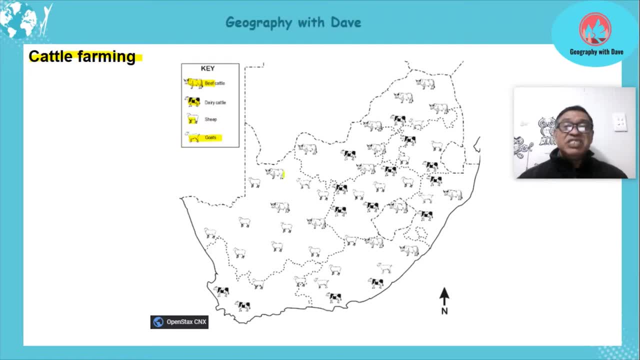 my apologies, I'm a bit thirsty today. all right, if you look at this, each symbol here, okay, cattle, that's beef cattle, dairy cattle, and then we've got sheep and goats and you can see how the cattle actually outnumber many things. all right, of the others, the sheep and the goats meaning that cattle farming, whether it's beef or dairy cattle. 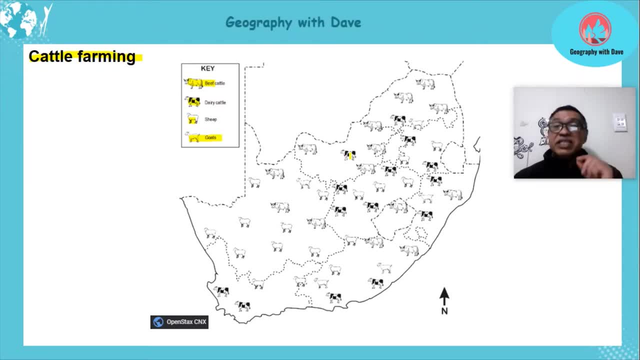 is done to a great extent in this country. all right, great extent, all right, more than any other sort of ones here, from the sheep and the goats, etc. okay, and another fact you will look at here, learners. if i highlight this section, all right, it's actually more towards the northeast and east. 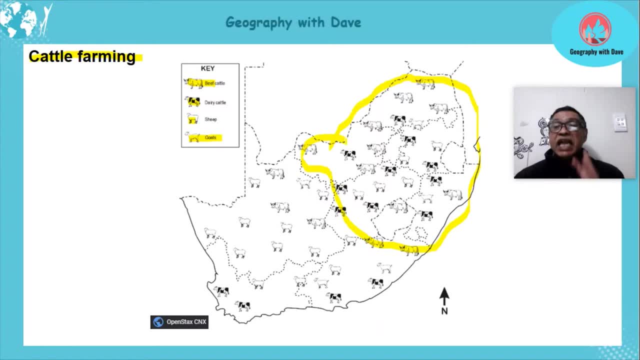 that's where the bulk of our cattle farming is done. okay, that's the bulk of it there in those areas. not that it's done in, not done in other areas it is done, all right, but the bulk of it is in that area. okay, let's go on. all right, let's start then cattle farming itself again. 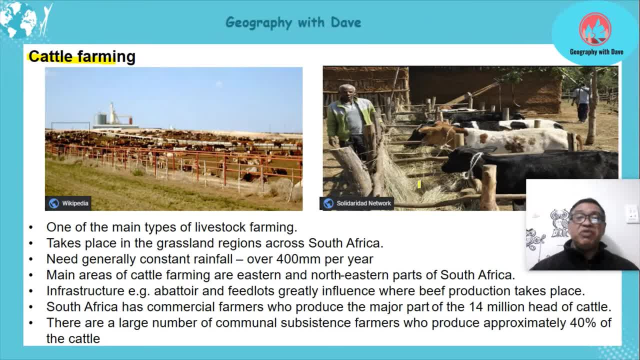 and move my face slightly. i'm sorry, i keep moving myself. i'm trying to be the center of attraction, not the notes, and i apologize for that. okay, is one of the main types of farming, of livestock farming. we've seen that on the map. okay, it takes place in the grassland. 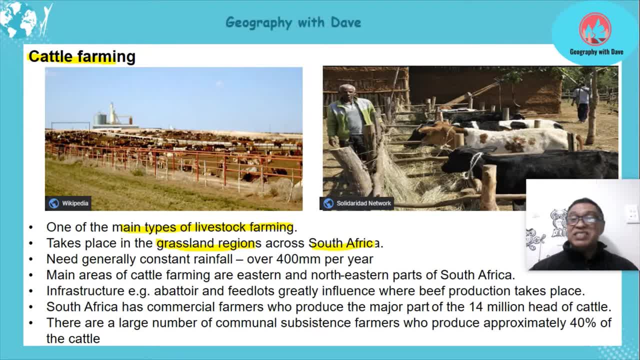 regions. all right, good pasture lands for grazing, etc. okay, and that's where the bulk of the grassland regions is found, in those areas highlighted where the bulk of cattle farming is happening. other things that we look at: it needs constant rainfall, over 400 millimeters per year, for the vegetation of grazing. 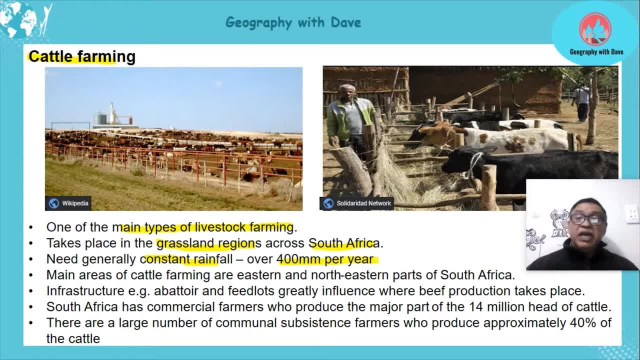 all right, and also for the cattle: okay, but most important, for the grazing etc. down there. we need the pasture lands- okay, main areas of cattle farming in the eastern and north eastern sections of south africa, as we highlighted there. all right, infrastructure. some of the infrastructure that we would need here is abattoirs and feedlots- all right, and this greatly influences where beef 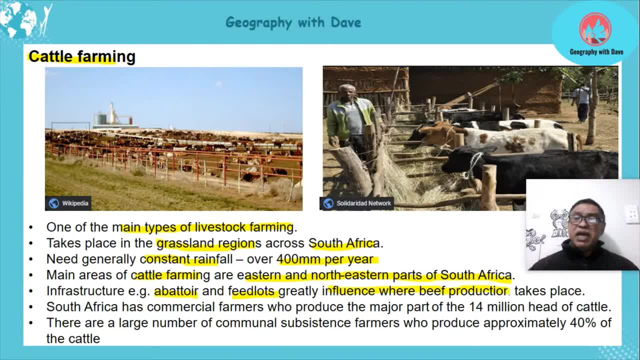 production takes place, okay. remember, cattle are heavy. try and lift one of them. okay, they're heavy, okay. so to transport over great distances is also a hassle and costly. so abattoirs and also feedlots for the cattle- all right. if it's closer to the cattle is better, okay, it saves a lot of money. so 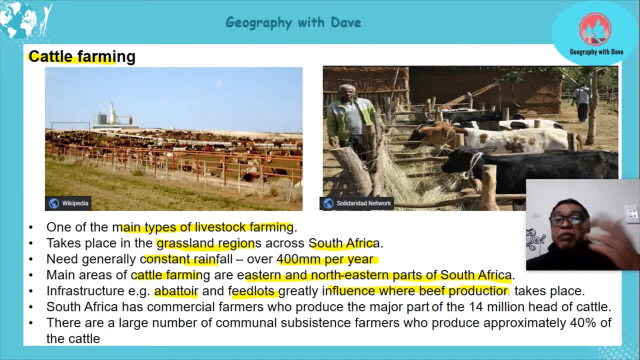 therefore, farmers also look at the abattoirs where they're situated and of course, more abattoirs will be situated to encourage cattle farming itself. south africa has boats as commercial farmers who produce major part of the 14 million head of cattle. all right, of course this is an approximate number. lots of cattle right, they play the biggest. 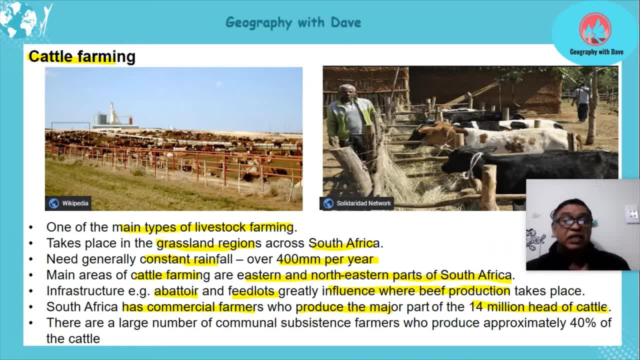 part in that, although they are smaller in number than the communal subsistence farmers. okay, now, when we look at that, all right, then there's a large number of communal subsistence farmers who produce approximately 40 percent of the cattle. okay, obviously, even though the number of commercial farmers will be smaller because of technology investment, large farms, etc. they hold a 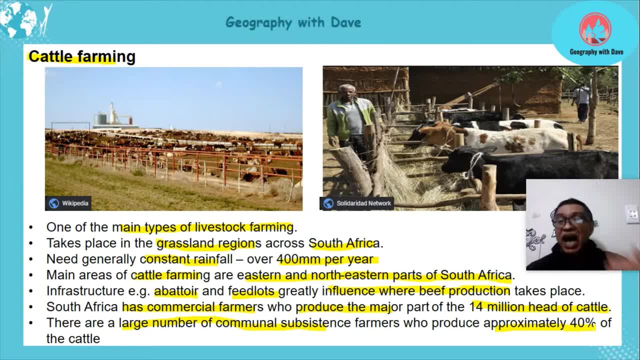 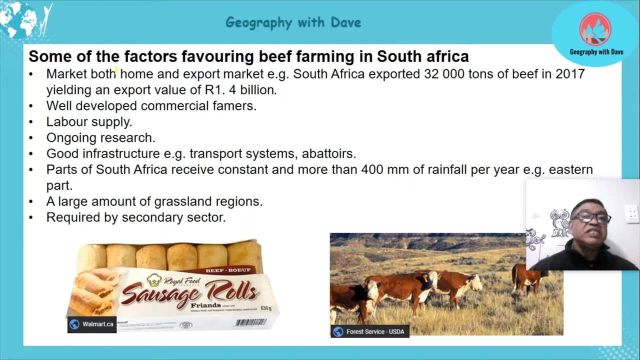 lot of cattle and their production is high, okay, whereas the large number of subsistence farmers, who produce approximately 40 percent of the cattle, okay, obviously, even though the number of farmers produce less, okay, per farm, all right, and therefore they'll have a lower number coming out, all right, but they all contribute, okay, right, let's go on with this. some factors favoring beef: 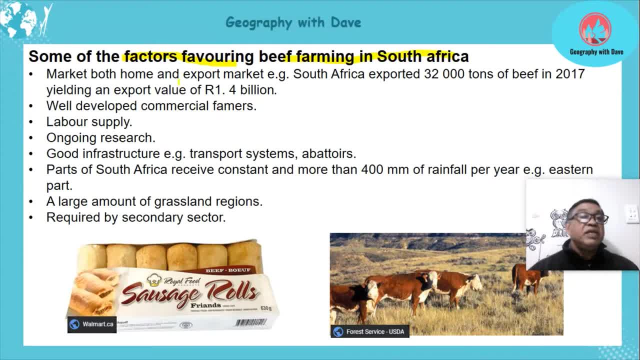 farming in South Africa. okay, now, market is important because, learners, if you don't have a market, why would we have commercial farmers? you understand farmers? all right, no one wants to buy it, it's not there. but the fact of favoring this, okay, is that beef is used. 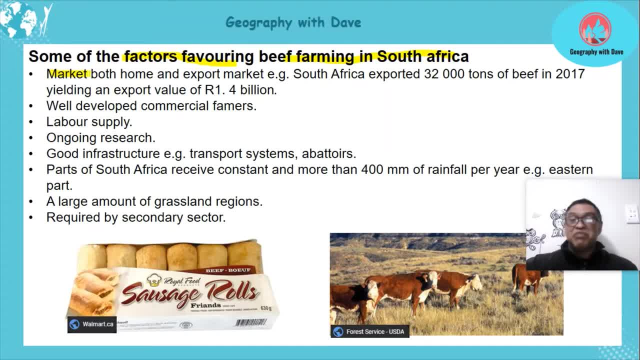 by the large population of our country. lots of people eat beef, okay, so it's used in the home. can we see you? we're talking about home and export markets now. home, but also the export market. we're sending it to other countries. all right, uh, we will notice that our consumption sometimes 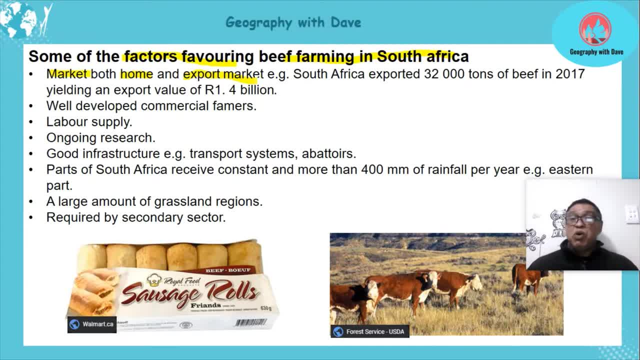 can be more than our production. that will reduce the exports, but over years, we do export. I will give you an example here: in 2017, 32 000 tons of beef were exported, all right, and the value of 1.4 billion Rand. that's a huge investment, all right, and it actually helps us in terms of a balance of trade, etc. okay, 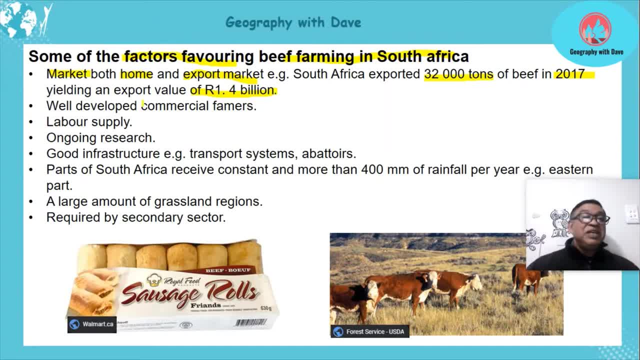 bringing in money into the country. all right. a good thing here is that we have well-developed commercial farmers. these guys are highly developed with machinery technology. you understand all these things that they are involved in, okay, but milking of the cows, etc. all this is happening. 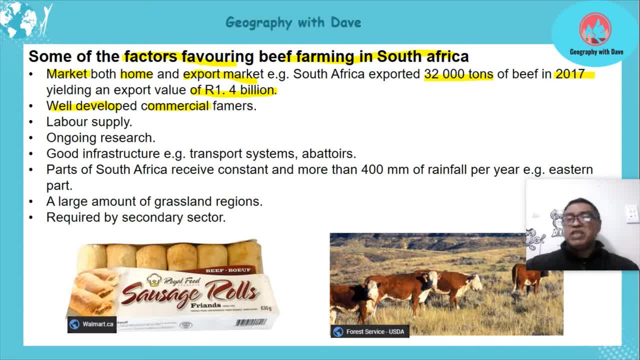 with these highly developed so they can have high production from their farms. okay, uh, we have labor supply, which is in abundance in our country. we have a high unemployment rate, so we have lots of labor supply. there's ongoing research. okay, that would you doing. various agricultural centers, research centers that are happening in this country. 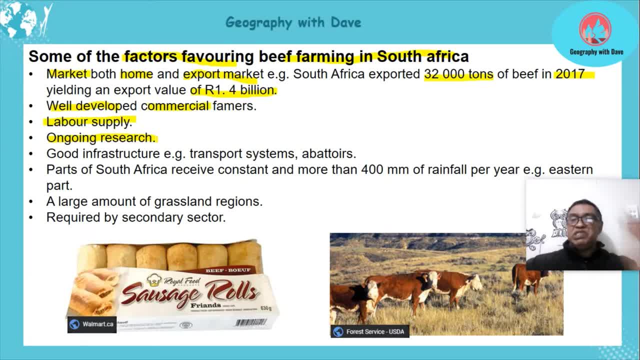 so we do have ongoing research which improves the beef farming, all right. a good infrastructure which is needed for transport- okay, i'm just giving you some examples here. good transport systems, all right, to move from the farm to the abattoir, etc. okay. or even if you're exporting, we have our 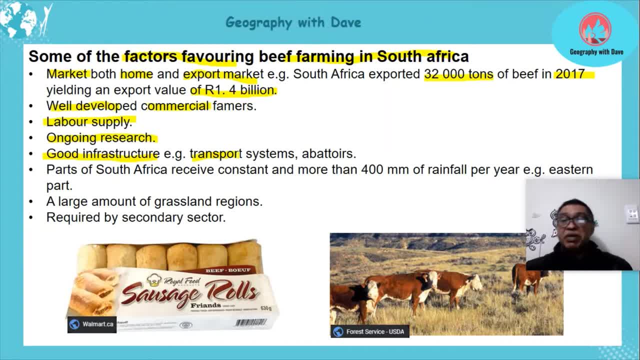 ports and whatever that we can export from or to neighboring countries. we've got good infrastructure leading to that, and then we have other things like a good system of abattoirs etc in our country. all right, uh, parts of south africa- and we looked at that- receive more than 400 millimeters of rain, for like the eastern parts, which allow for more productive. 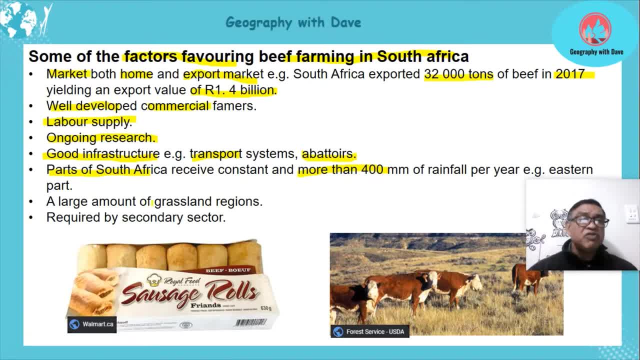 beef farming and we also have a large amount of grassland regions, as we've seen. this is one of the factors. you can see these cows enjoying them- you can see meat meat here here in several parts- and enjoying themselves on the grassland regions here. all right, which gives pasture lands, etc. for the 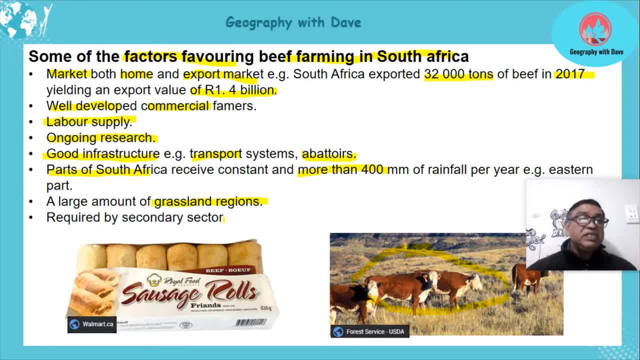 cattle. all right, important. and another thing: it's it's required by the secondary sector, so it's favoring. production is increasing because of the secondary sector. now this is making me a bit hungry, but i lived it till after the presentation. all right, i'll get my family to make some of this. 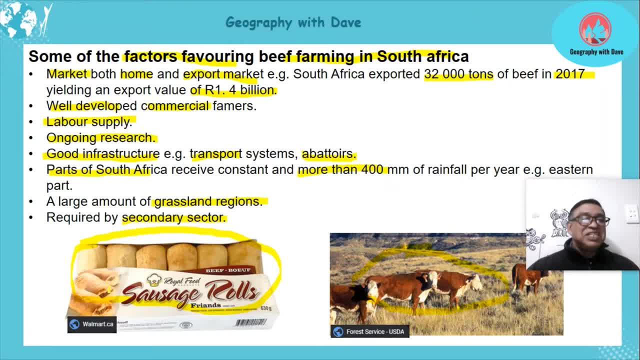 for me, okay, right. for instance, sausage rolls, beef sausage rolls- whoa, they look nice, okay. so what you call it is, uh, this raw material- i'm gonna call it a raw material, all right, uh- is used to make or manufacture the pies. in fact, the skin of the cattle is used even for leather. 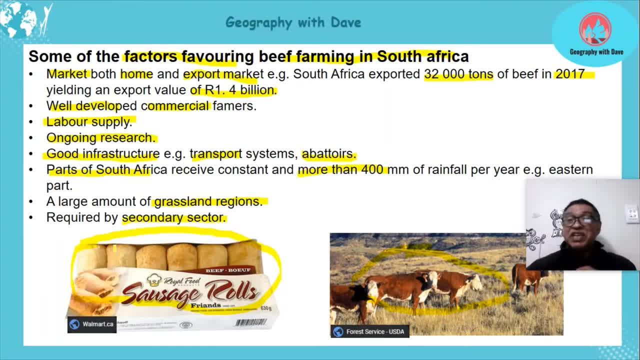 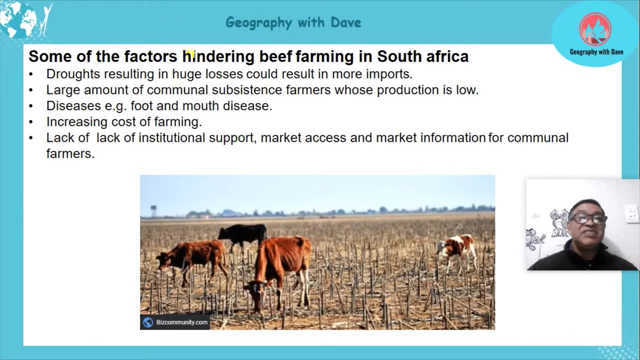 okay, so because of that, it's a factor favoring production of it. okay, some factors that hinder the negative factors towards beef farming: all right, a huge problem here, learners- droughts, okay, uh, it actually causes losses in cattle, all right, and result possibly in more imports, because now we can't export if there's a drought, we have to buy more. 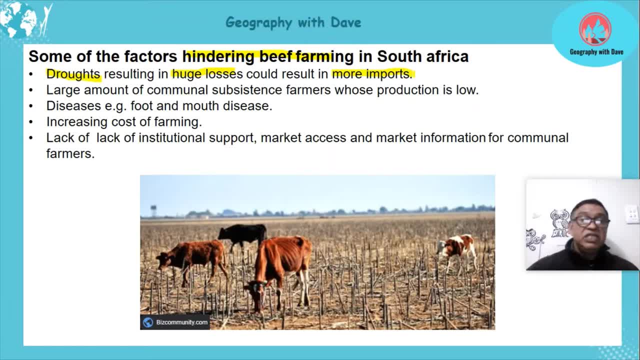 and we can't export. if there's a drought, we can't export. if there's a drought, we can't export. if there's a consumers in our country, all right, and you can see this picture of a drought. look at the cattle here. it's a sad story. all right, very thin, etc. and sometimes farmers- what they do is as the season. 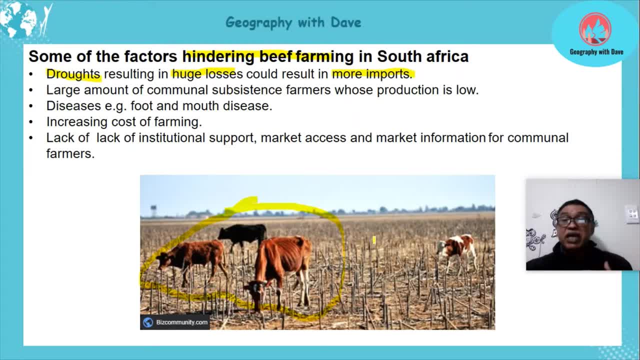 is progressing and the drought carries on, okay, then they slaughter their cows- okay, and- and sort of try to sell them or freeze them or whatever, so at least they can have more meat instead of the cows ending off like this. so it's a factor that is totally negative and it if 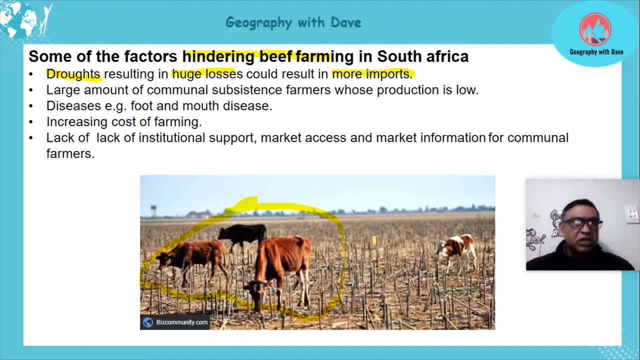 affects our country's lands. it affects our country a lot. all right, the large amount of communal subsistence farmers whose production is low. okay, now, this can be a factor, a negative factor, all right, in terms of producing. okay, uh, beef. okay, to a large extent, because their 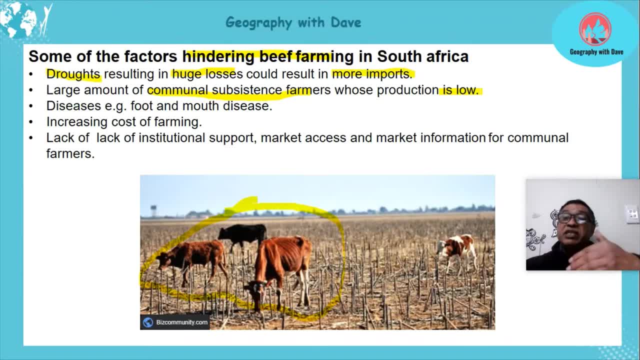 production is low, and especially when we're starting to get the consumption being higher than the production. i'll talk about that later. all right, this does not supply as much. okay, so we need to government, or whoever needs to be involved, in order to educate subsistence farmers, increase the. 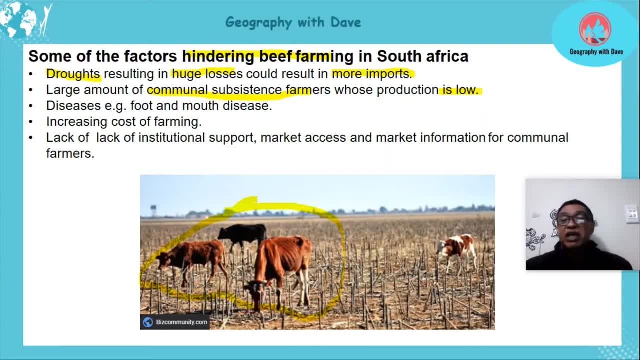 production, bring them on the commercial basis. okay, that could help, all right. then we have other things like diseases: your foot and mouth disease, which is quite serious when it comes to cattle- all right, it's quite serious and it actually kills the cattle. we had mad cow disease, that starts. 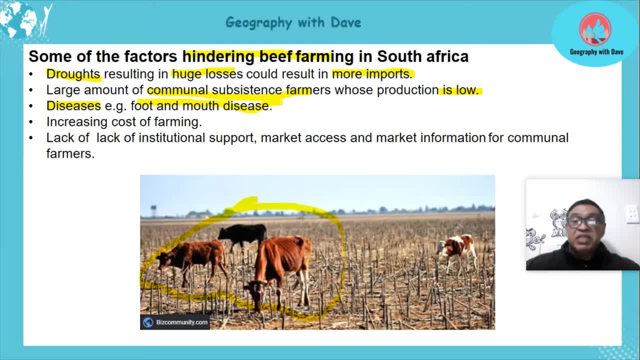 spreading. not as much in our country, all right, but these sort of illnesses that come in foot and mouth is more common, okay, increasing costs of farming, which makes it difficult, cost increase. you know your father and mother or guardian, all right, is complaining whoa the price of this and that. 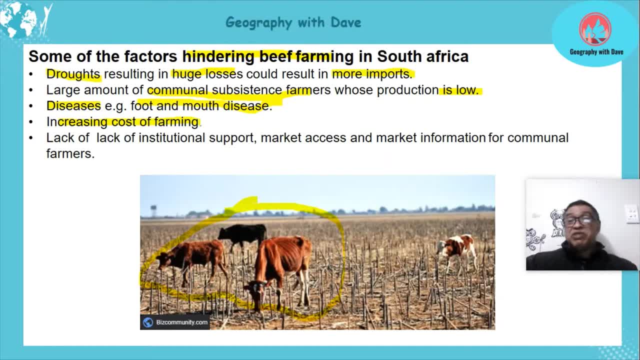 is too much, you understand, you can't afford it. remember the farmers also: their costs go up, okay, and they can't drastically increase prices, okay, because then people may not just buy, okay, so that is a factor that in that lack of institutional support- okay, i'm gonna talk about. 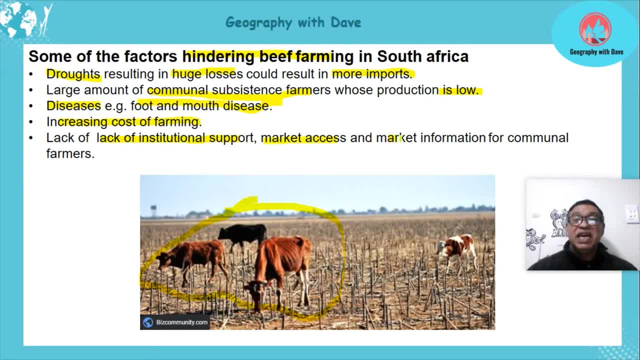 this now. let's go through this first: market excess and market information for the communal farmers. okay, we're farming in a community subsistence level, etc. and that's what i'm saying. it's a lack of support. this is a lack of support, and that's what i'm saying. it's a lack of support. this for. 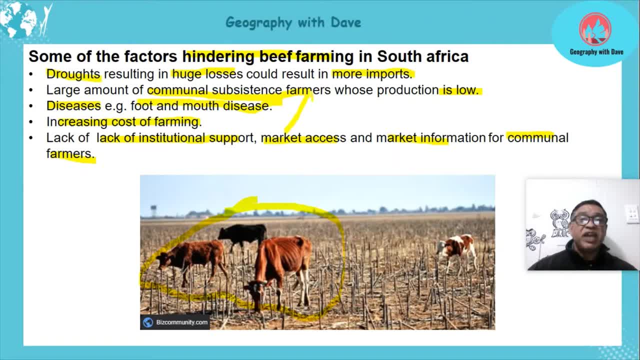 the community subsistence level, etc. and that's what i'm saying. it's a lack of support, this for the community subsistence level, etc. and that's what i'm saying. it's a lack of support. this for maybe related to this factor, okay, but there the production is low- and also the lack of support. 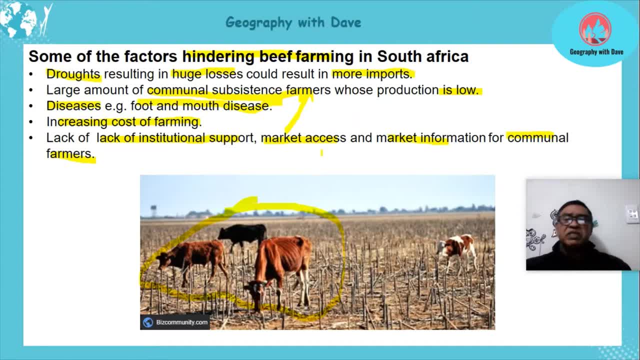 for them from the institutions, from government, all right. they don't have much access to the market, okay, and in fact, the market information of what the market is, how can they produce to sell to the market? all right, and if we use these factors, learners, all right, where we say to them: 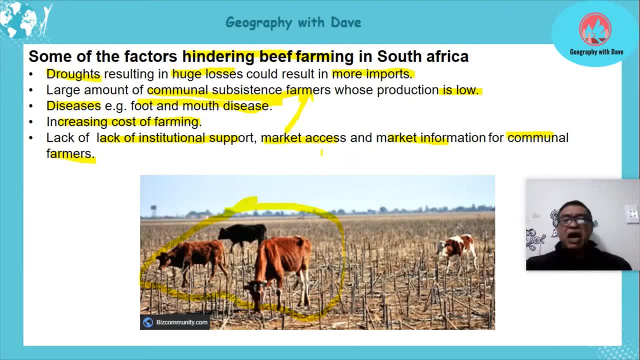 you know what, guys? if you can sell, we introduce you to the market. okay, this is what can happen. you can earn your money, improve your quality of life. we're bringing people to advise you, to show you that we could change these communal subsistence farmers. you understand, because 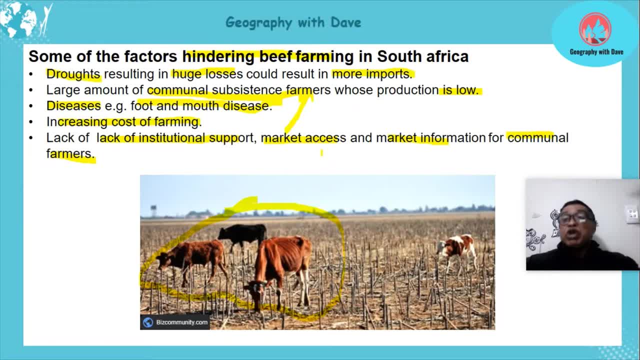 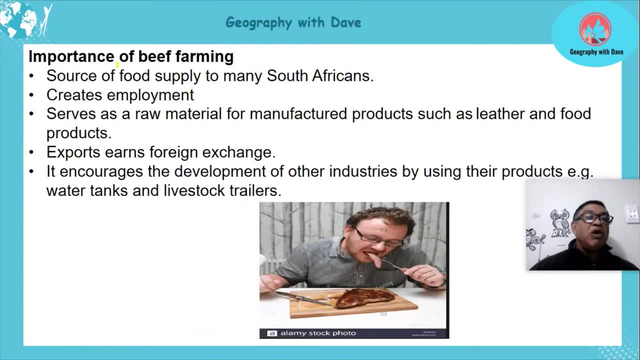 it benefits them and it benefits the production. okay, right, let's go on the importance of the beef industry. it's a source of food supply and you know you will carry on the concepts like your proper food supply. you understand where you don't really have. you need food security. 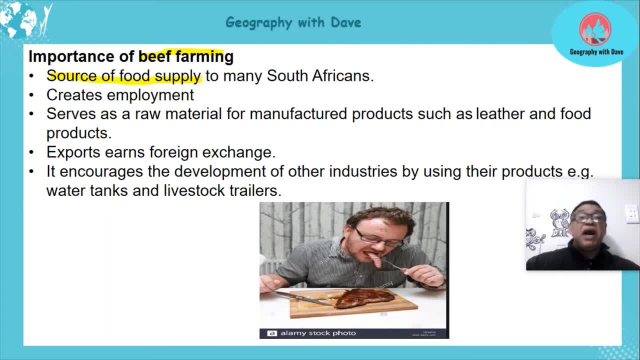 okay. in the country. beef can play a big part- the production of beef, enough beef, okay- and it's a source of food buying for many people in the country. it's quite a favorite food for many people. you can see this guy. i decided to put a picture. why do we keep on being with the serious? 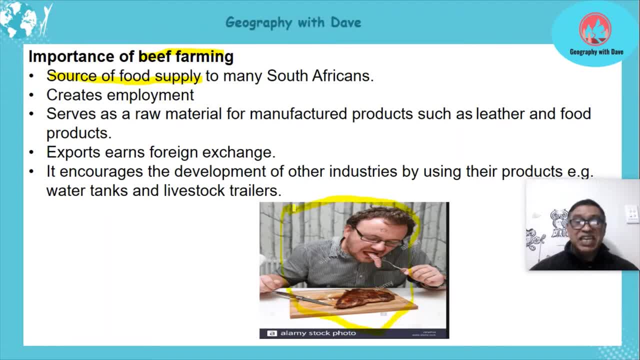 stuff. you can see this guy here. oh, he's eating this steak. can you see this nice steak down here? whoa, all right, uh, he's enjoying it. so it's a food supply which is important. it does create employment- people working on the farms, all right, uh, and all other areas remember. 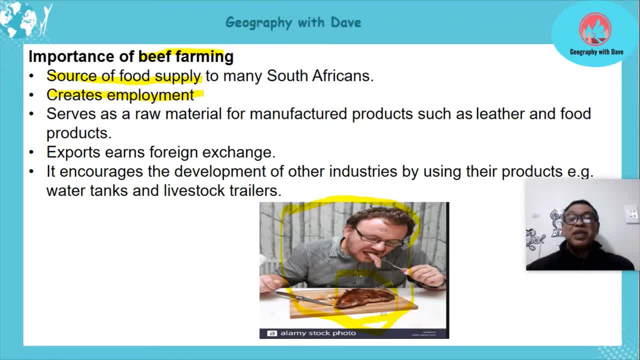 when we say creates employment, we don't only talk about the farm. all right, these products are taken and manufactured. so indirectly it's playing its part in the secondary industry. then we have restaurants, okay, in the tertiary sector, all right, where it's creating employment also. so it has an direct on the farms and indirect it supplies employment or creates employment. 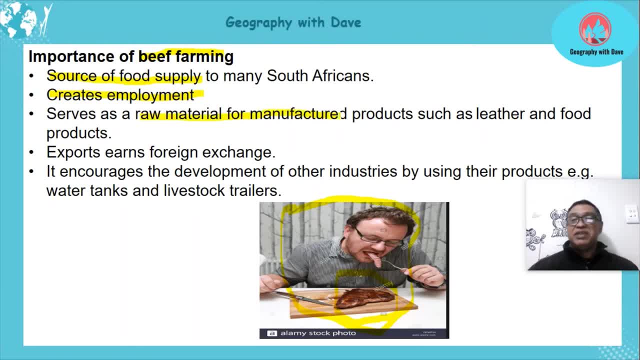 serves as raw material for manufactured products- okay, important, all right- such as leather and food products as this, sausage rolls and whatever. oh, i'm really getting hungry now. all right, so it serves as that, all right. it earns foreign exchange because we selling it to other countries, we're getting the money in. 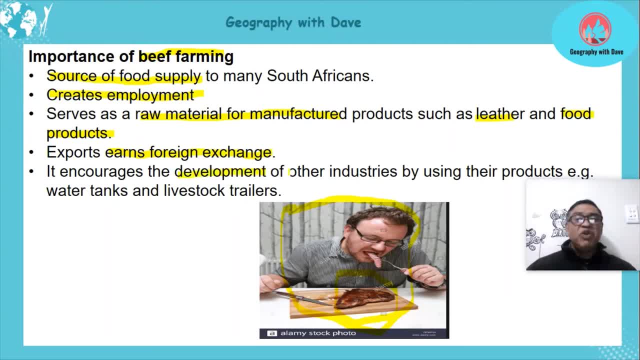 and it encourages the development of other industries using their products. example: water tanks and livestock trailers. i just gave a few. so the commercial beef farmer needs this equipment. he needs the water tanks, all right. he needs the livestock trailers to transport his stuff. now these companies who are producing them, all right, they come up because of the beef farmer. 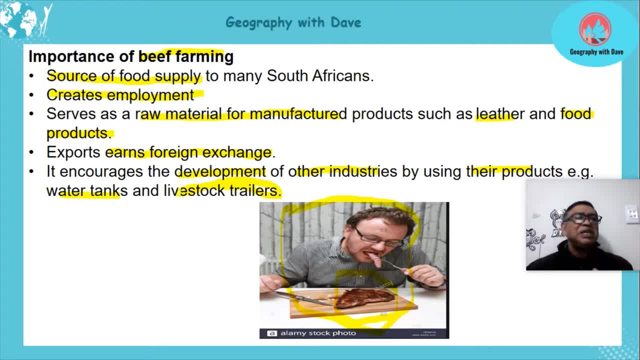 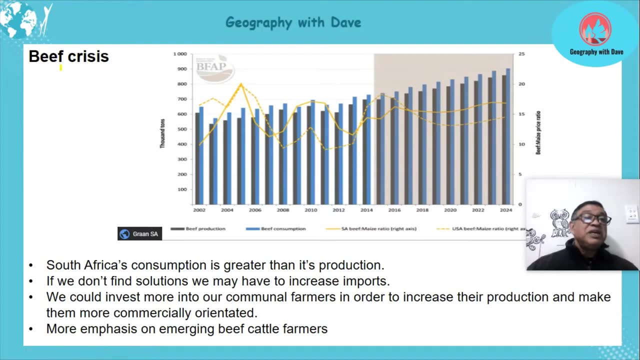 okay, can you see? so it's such an important thing beside the economic development. all right, the specifics to the economic development. let us- i'm going to switch the slide. this guy eating the steak is making me very, very hungry. all right, let me go forward. all right, now there's gonna be a beef. 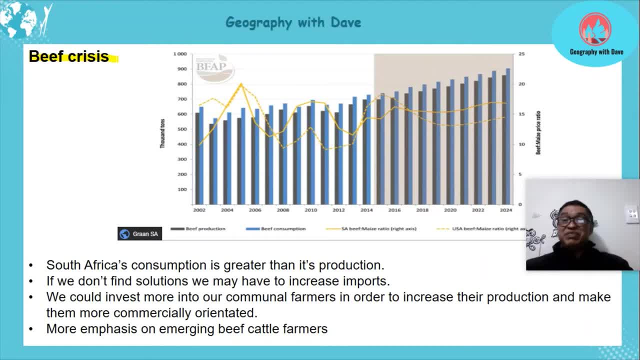 crisis. i call it the beef crisis in the future. it seems all right. now we're gonna look at this graph. the blue talks about the dark blue talks about the production. the lighter blue talks about the- uh- beef consumption. can you see that? i think people call that the navy blue way, you see? 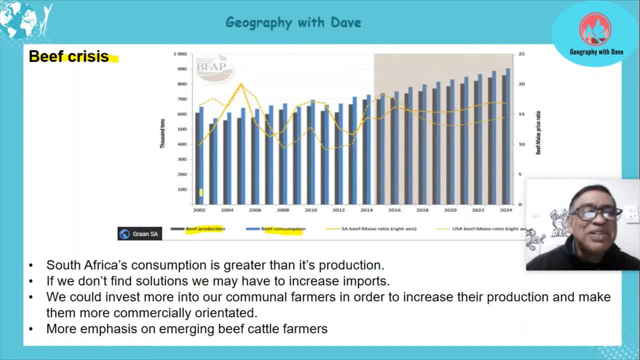 geographers don't know their colors, right so, but these two represent that. can you see? now, what do you notice? learners, in all these sections heading from 2002 to 2024, the production is less than the consumption. that is a problem, learners. consumption is greater than the. 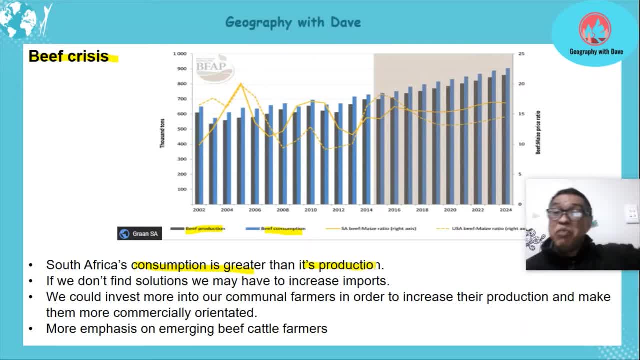 production. i put it the opposite way. that means more people want beef than is being produced and that's a hassle and we need to find solutions because there's an export market out there. all right, if you don't find, we'll have to increase imports. we want to export. we have a market out. 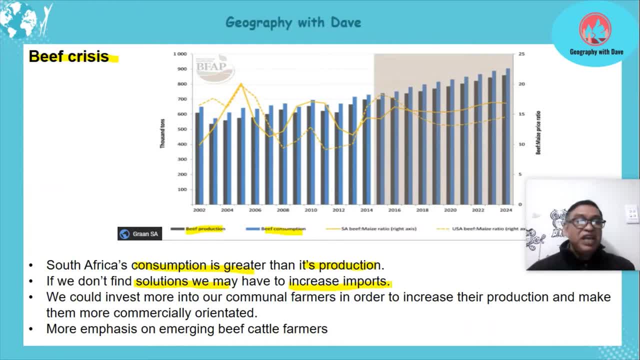 there. let's not lose it. so we need to find it. we need to invest more time and effort and finance into it, and one of the ways: invest more into our communal farmers in order to increase production and make them more commercially orientated. okay, more small-scale farmers, etc. that we could help. 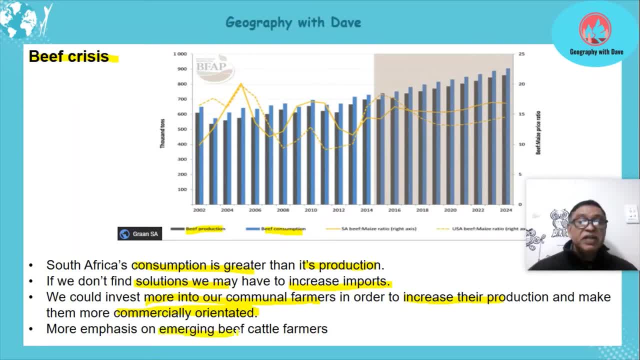 okay, like this emerging beef cattle farmers- all right, i should say beef or cattle, but i'm trying to over emphasize my point there. all right, so be farmers. all right, we should, these emerging guys who lease land right to farm on. we should actually support them and encourage more of these emerging farmers, because it's going to be good, the production will. 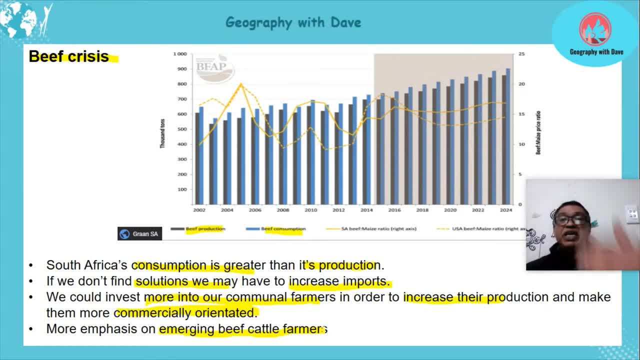 increase with enough food in our country, plus, we can export, all right. so that's the crisis. the beef crisis, okay. well, i hope we don't reach that where the beef prices go up and then it's going to cost us so much, okay, and i'm going to lose out on my beef. let's look at the next major. 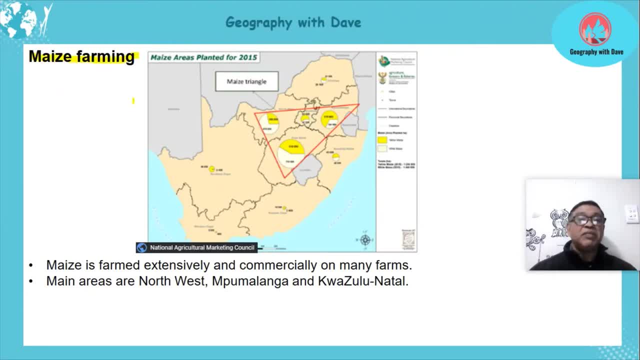 one is maize farming. all right now. maize is extensively farmed and commercially on many farms. maize is a huge product in our country- huge. i'm going to go further into it and tell you how huge it is. all right, of course, our main areas is around here. all right? uh, we look at the places like the northwest and pumalanga. 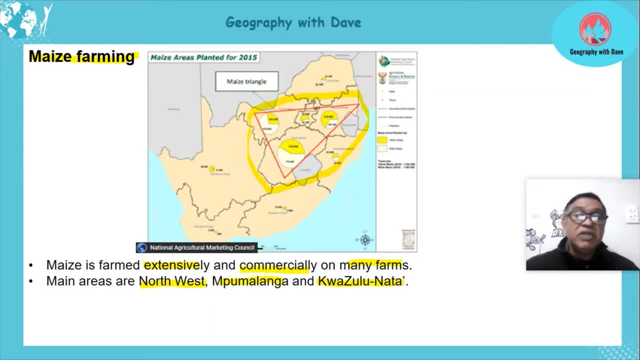 big areas for maize farming- huge right now, that it's not farmed everywhere else, but it's much smaller. they, these have, these areas, have the conditions for farming of maize. okay, so it's that area. all right, let's go further, all right. now i want to. 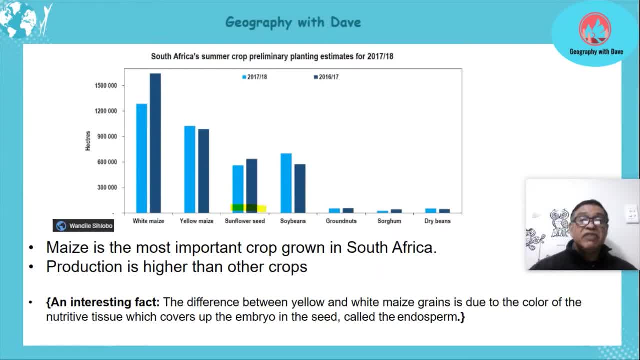 show you something here. it's compared to others like sunflower seeds, soya beans, ground nuts, sorghum, dry beans- all right, look at maize here. look at maize. all right, this was for 2017.. 2018, all right, okay. so if we look at it here, the light blue is for 2017- 2018. 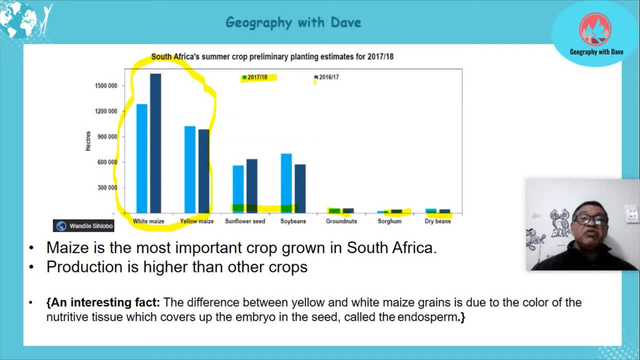 and, of course, the dark blue. i like to call it. the dark blue is for 2016- 2017.. all right, but that's not the main issue here. the main issue i want you to focus on is look at how much maize is being produced compared to these other products here. that's massive difference between. 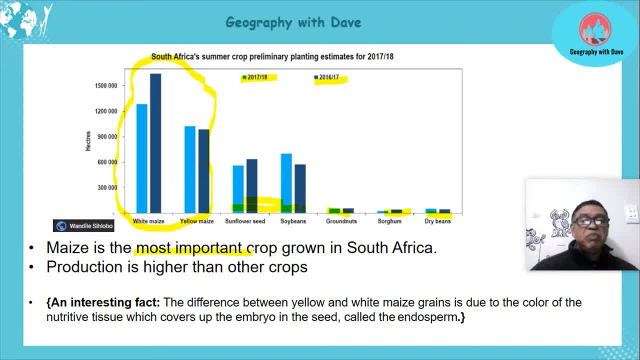 them. so maize is regarded as the most important crop grown in south africa. the production is higher than other crops. you can see it here: lens high. okay, just a matter of interest. all right, this is not part of your curriculum. okay, but i thought you need to know because we come up with 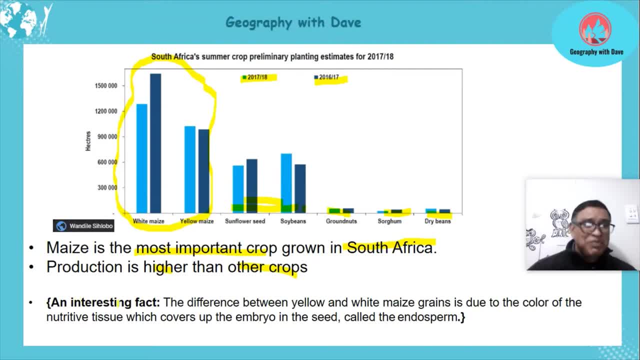 this word: white maize and yellow maize. so just as a point of interest, the difference between yellow and white, you would have guessed it is due to the color of the nutritive tissue. okay, which covers up the embryo. i've learned about the embryo in the bean also, or in the maize rather. 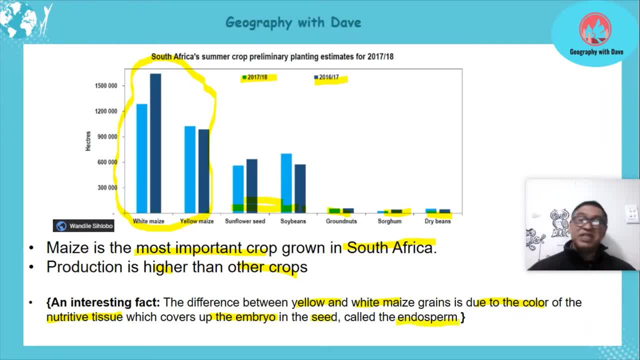 in the seed, called endosperm. interesting, eh, but anyway, that's not part of your curriculum. so if anybody asks you a job for, tell me the difference between yellow and white maize, you know, just tell them about the embryo and the endosperm, whatever. it's quite interesting, all right? okay, let's go on. so we learned it's the most important. 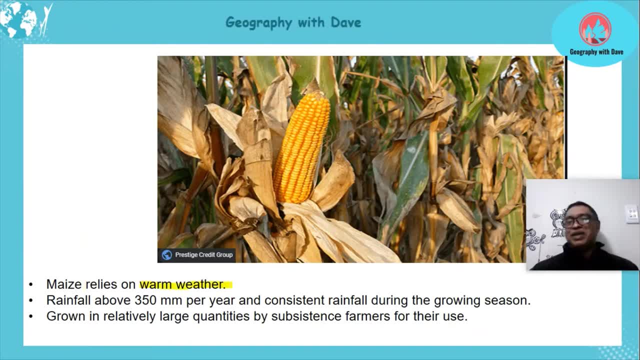 crop maize, relies on warm weather. okay, that is why these regions rainfall above 350 millimeters a year and consistent rainfall during the growing growing season. what what we mean by consistent rainfall? this 350 millimeters of rainfall mustn't fall on one day and then doesn't fall again when it's a growing season. it must be spread out. 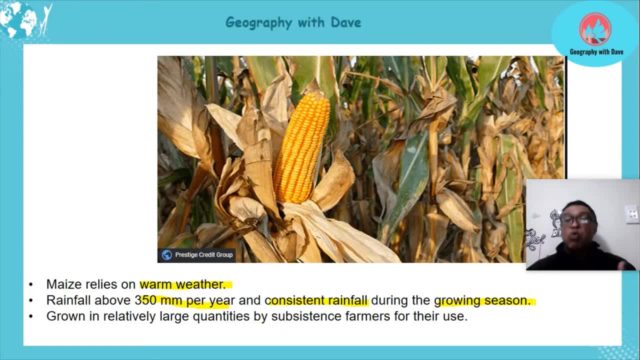 during the growing season, allowing it to grow properly. okay, right, it's grown in relatively large quantities by subsistence farmers, also for their own use. all right, it's growing large quantities by them also. you find maize being grown on a substance level because it's a staple diet of. 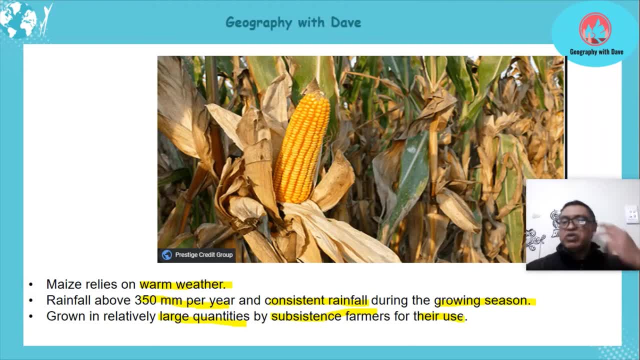 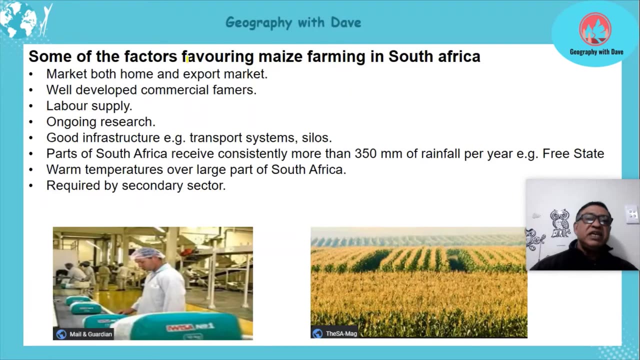 africans. we all use most over 95 or 98 or 99 of us use maize in our country. all right, it's quite a common uh food. okay, some factors favoring maize farming as a gain in the, in the other ones, and as i go through some of these list learners, i'm not gonna waste uh your data because we discussed. 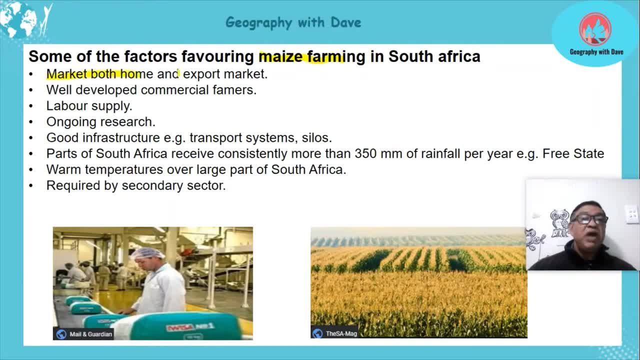 it already. so when it �ren�� 좀ken ghinais quím để mình khça corps h pointer to agenda because we've discussed it already. so we we know it's both home and export market. i'll show you some figures later, okay. 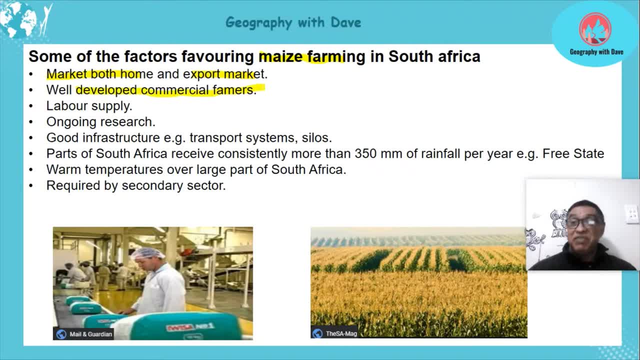 then well-developed commercial farmers, okay, factor favoring, okay, you can see it here. whoa massive maze. all right, the labor supply: you know already, right from the uh previous one on beef farming: you need people to farm and it's linked to the secondary sector also, where these 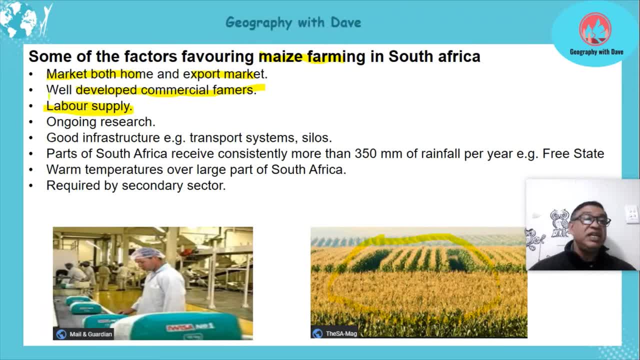 people are producing the maize and the tertiary sector, ongoing research, like beef farming- there's lots of research, improvement of seeds, etc. for growth, right fertilizers, all these things and again good infrastructure in terms of the transport systems, transporting it through the country and wherever it needs to be exported, things like silos to store the grain. all right, the maze all. 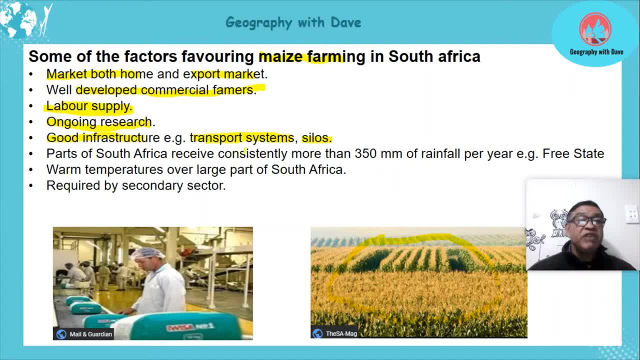 these things are available and you see that parts of south africa receive consistently more than 350 millimeters of rainfall. it must be consistent, all right. example: the free state for the growing season. it's good. so we have quite a significant part of south africa as situated in those areas. 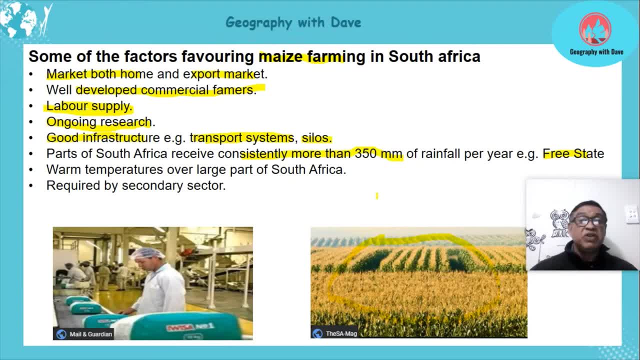 like the free state, that produce that have the good, suitable rainfall for growing and, of course, warm temperatures over a large part of south africa also to allow it to grow properly. we also learned that it's required by the second that he said the same, like beef farming. he has an example in wisa. can you see? 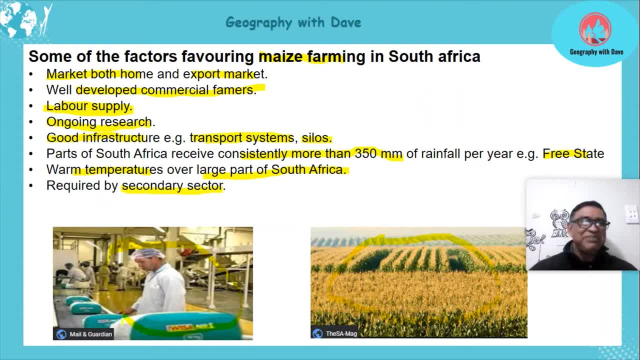 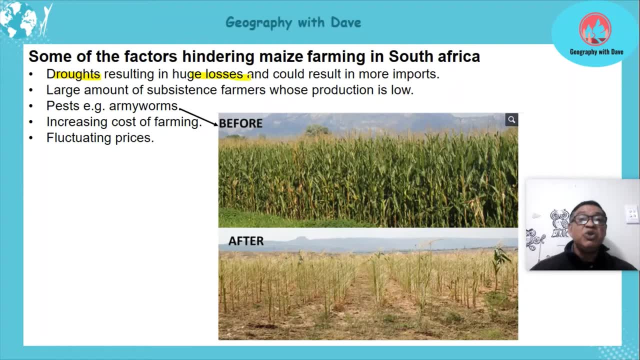 base meal being produced and packaged. okay, then we go to factors hindering once again droughts. huge losses could result in more imports during those drought periods and we have a large amount of subsistence farmers whose production is low. you've done letting beef farming and you know, less is produced. we have piss like the army worms. whoa, they're dangerous. 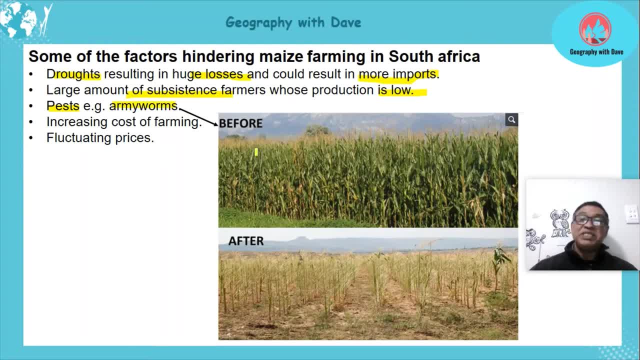 they are dangerous. look at this little uh picture here. all right, look at here. all right, this was before and this was after the army worms went through the field. that was before, that was after. okay, ah, sorry, let me get back to that slide. okay, and, of course, increased costs of farming, which makes it 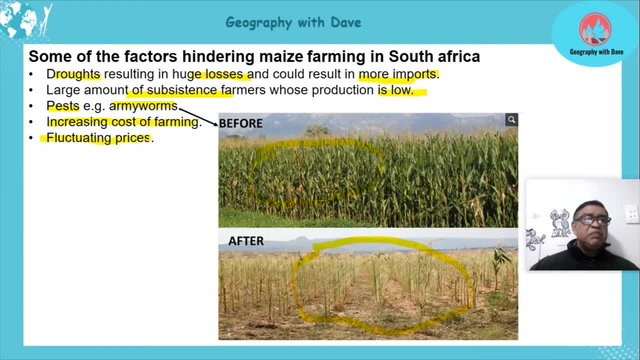 expensive for the farmers and fluctuating prices. fluctuating prices, you know it's hard to plan how much to farm. what's the cost going to be if prices keep going up and down all the time? all right, it makes it difficult for the farmer and when it goes, when it's expensive, farmer produces and suddenly the prices go down and he's invested. 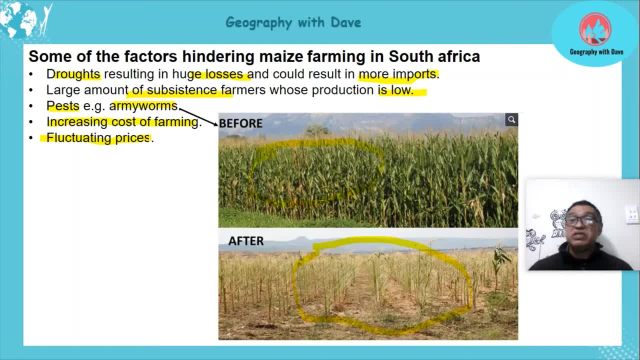 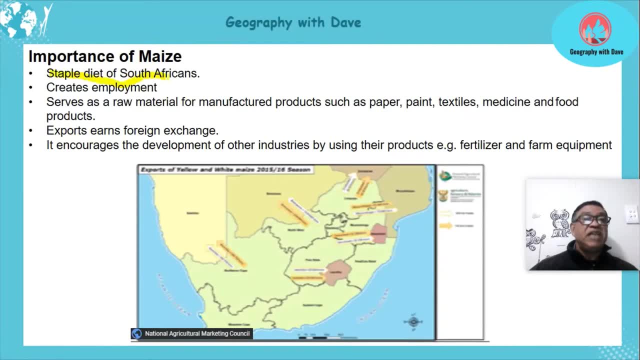 so much. all right, now he's at a loss. okay, okay, importance of mes. it's a staple diet for most south africans. they eat it. all right, your Pop, etc. when you're having that brine, okay, pop and fleece and chakka, laka wool. I'm now getting very hungry. how i just hope. 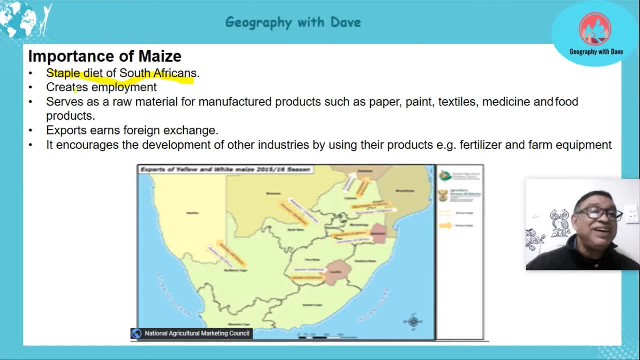 i can manage to finish this lesson, all right. okay, it creates employment. we know that. as in employment, its a staple diet. you know we eat it every single day and jerkalaka wool. okay, important importance of this. it's a staple diet for most South Africans. they eat it all- uh, your pup, etc. 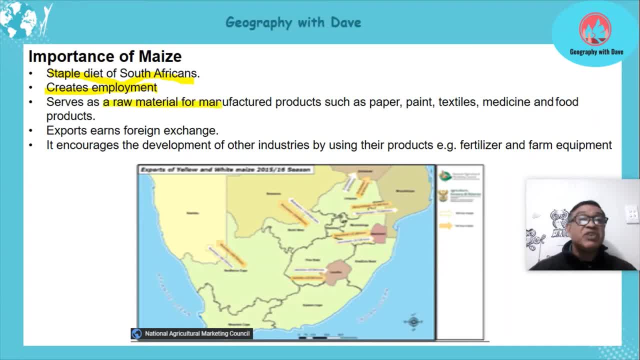 that, as in beef farming, again it serves as a raw material. i'm sorry i'm going over this again, but of course the examples will differ for manufactured products, paper, paint, textiles, medicine, food products- okay, in all this is used, it earns foreign exchange. all right, look at the. 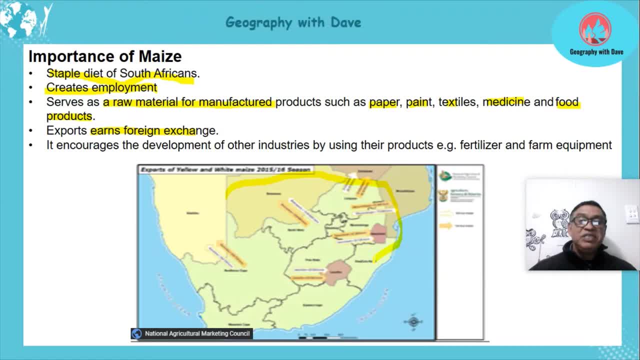 places that it go to. all right, all these different areas it's going through, so it serves so many other countries. we export to them, so it brings in a lot of money and, of course, as in beef farming, with maize, development of other industries. example: your fertilizer, your farm equipment. 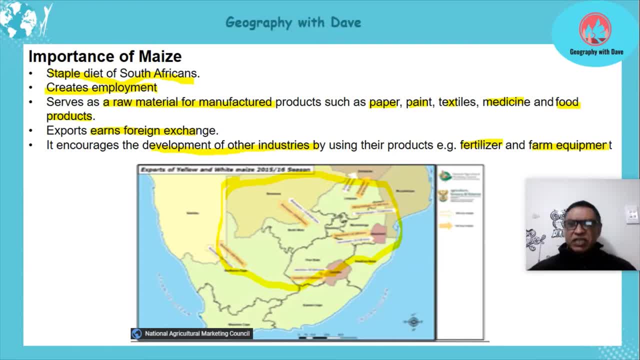 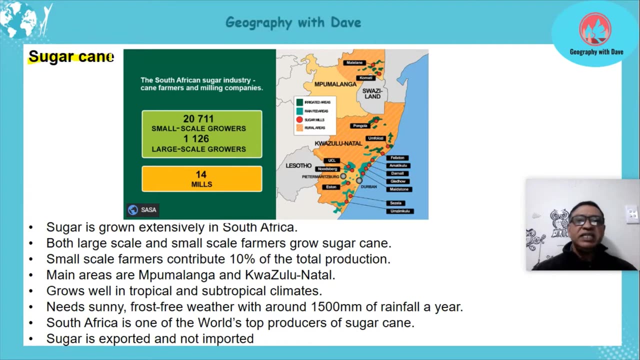 all those industries develop to a great extent. all right, because it's needed by this- the large production of maize by farmers. okay, right, let's go on sugar cane now. we look down here, we see it all along the east. the climate makes it all right. we can see that it's grown extensively in south africa on a large level. all right, there's large. 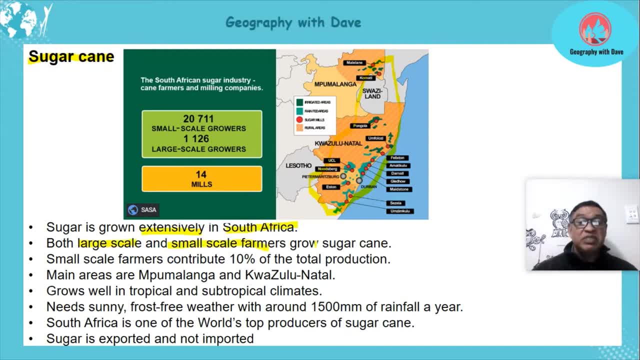 scale and small scale farmers that grow sugar cane- okay, even your small scale farmers grow it for us for a commercial basis- okay, so it doesn't. can you see here there's twenty thousand seven hundred and eleven small-scale farmers- okay, and there's 1 126 large scale farmers. so it's a lot of small-scale. 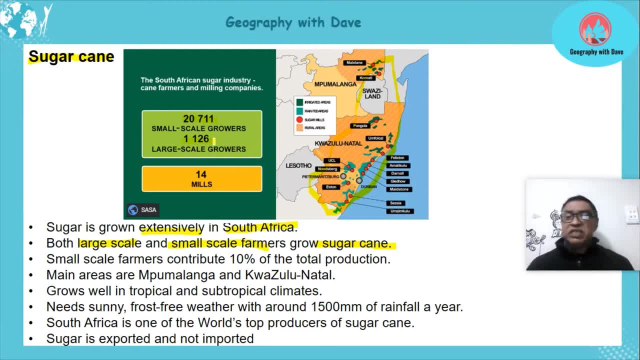 farmers. obviously, this one thousand one hundred and twenty six learners will produce far more than the small scale, because their production is high, all right, their farms are massive. if you come along this areas here, you will see the large sugarcane farms that are found across this area. 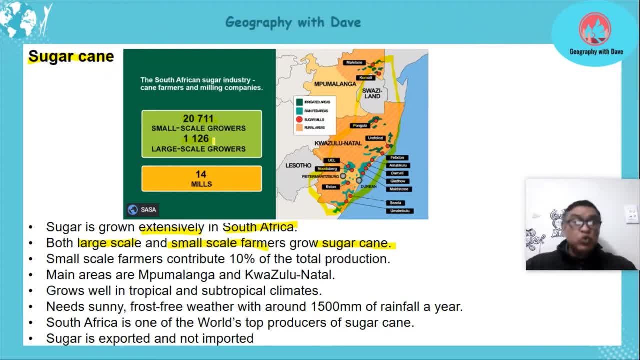 hectares and hectares of land. all right, it's huge, okay, but the small scale farmers contribute 10 percent of the total production, quite significantly. land is quite significant, all right, but you must think about those 1126 large scale farmers. they must be whoa rich, rich. 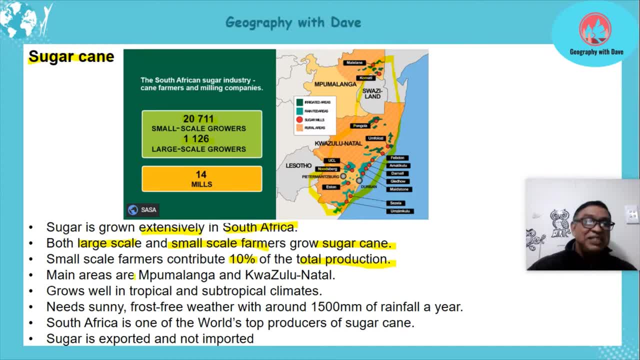 people. all right, producing so much main areas in pumalanga and kwazulu natal is massive. okay, the sugarcane chicken grows well in tropical and subtropical climate and we know along the area here, okay, in kwazulu natal, subtropical climate, so the sugarcane just grows all that time. okay, it needs sunny, frost-free weather. 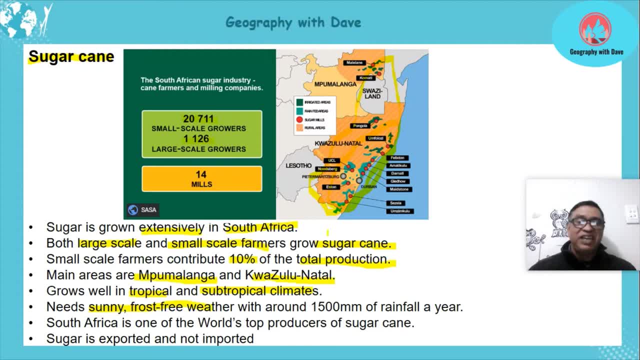 that happens. yeah, we don't get frost along this area, with around 1500 millimeters of rainfall. it needs a lot of rainfall, sugarcane- and i don't know if you bought any sugarcane like that when you travel around these areas and you bite it, you actually get the liquid, so it requires a lot of. 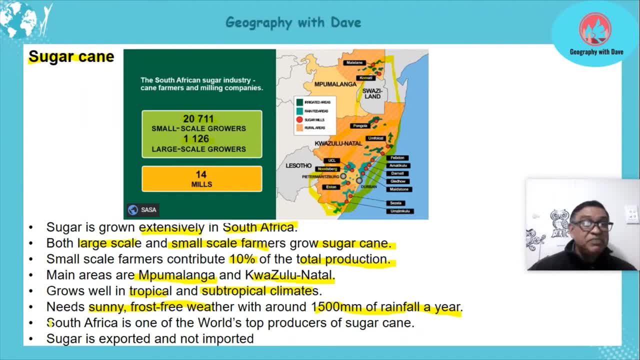 water. all right, it's. south africa is one of the world's top producers of sugarcane. all right, it's one of the world's top producers. so we're quite massive at this. generally, sugar is exported, not imported. we have enough sugar. that shows we're very sweet people. lots of sugar in our country. 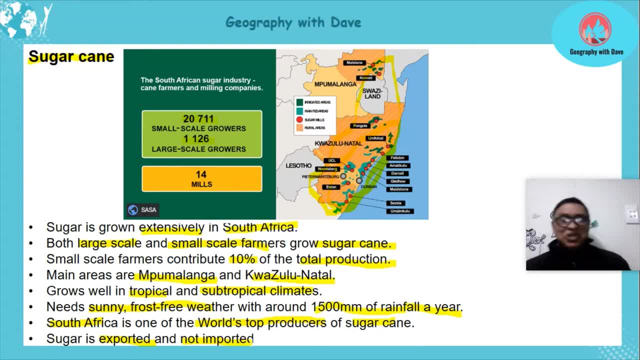 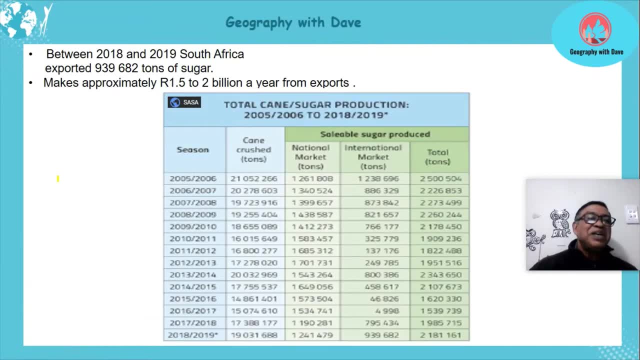 sweetness of south africa. okay, so we have all the sugar in this country, all right? okay, look at this. between 2018 and 2019, we exported 939 682 tons of sugar whoa- set the figures properly, all right, and one made approximately 1.5 to 2 billion rand. 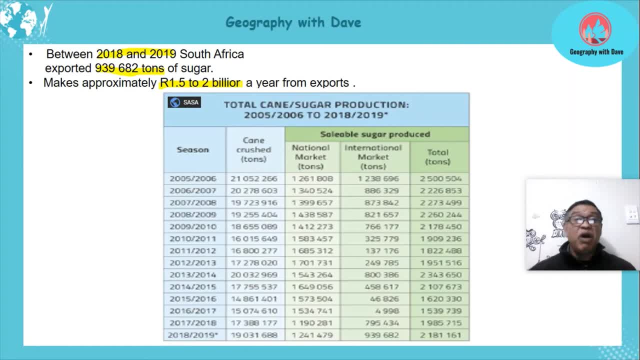 okay a year. that's what you make a year. for hours it can be even higher, but that's just the average. okay, a year from exports. massive amount of money, all right, from exports. i just used those figures there and i can show you here, all right on this graph, on this table, rather the amount. 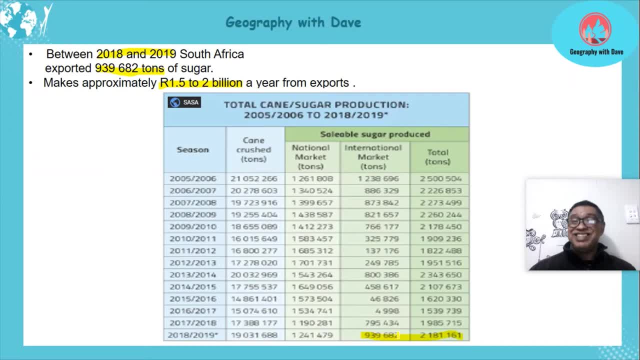 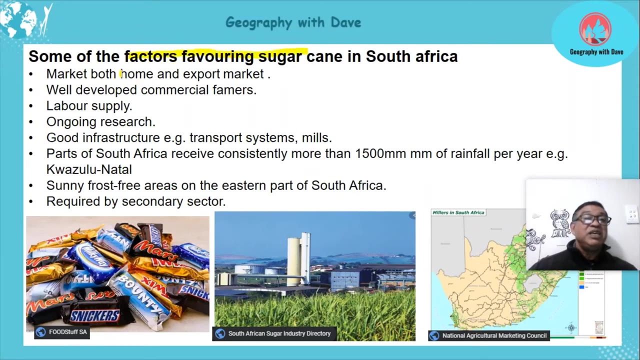 that goes, made this international market in tons, massive amount. all right, let's go on. and why we're not going on? yes, some factors favoring, and again it's a lot of the same factors. it showed you the amount of money it's used at home and the export market. okay, right, 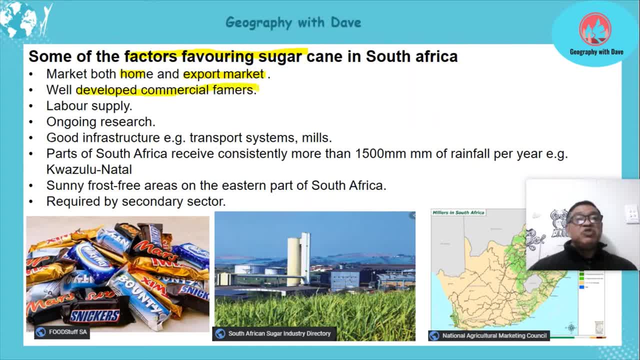 a well-developed commercial farmers. you saw those 1,100, some odd farmers compared to 20,000. they produce 90% of the sugar. it needs labor supply, as again I said, directly on the farms in the secondary activity where you're making those lovely chocolates. 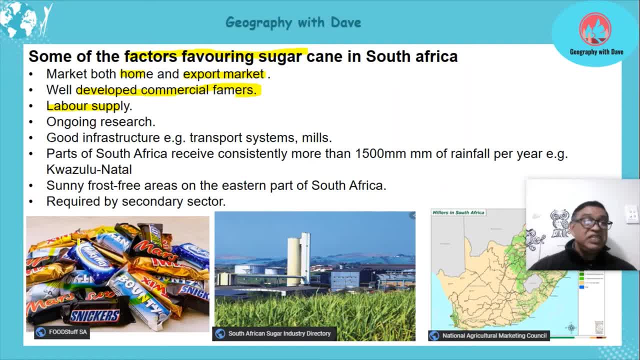 you understand, they get manufactured. all right. now I'm feeling for sweets, right. I'm really suffering through this presentation of all the good food. okay, so, uh, chocolate, etc. all right. so labor supply- supply there and the tertiary sector: okay, ongoing research. that's happening all the time. we're one of the world's large production or producers of sugar, so research is encouraged. 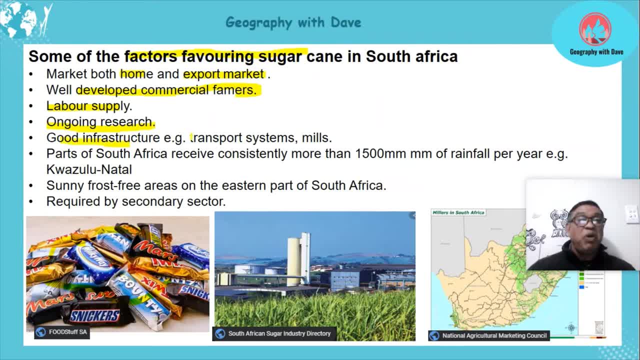 a lot good infrastructure. transport- okay, we, even here. we can pick on the port that's found in Durban, you understand- where we can send our sugar off by ship. okay, that shows it becomes sweet chips also, all right. all right, so we send on our sugar quarrows. can you see there's a sugar mill? yeah, okay, that's there. 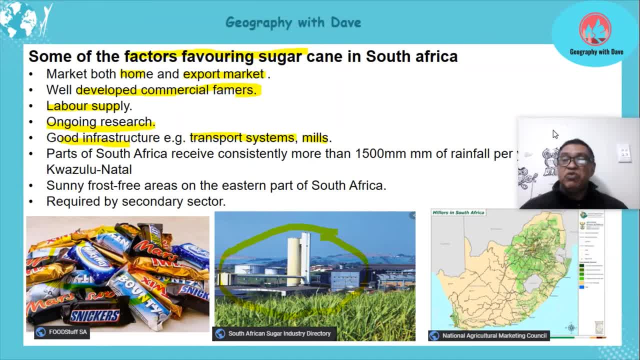 and I'm gonna move this STEVEN measure j з j. hey, Love it. bye, bye, bye, bye, bye, bye, good bye, bye, stuff. okay, i'm looking at the chocolates. let me switch quickly again, right, uh, but i have to explain some stuff. sorry, so i have to stick my torture of those chocolates. all right, parts of. 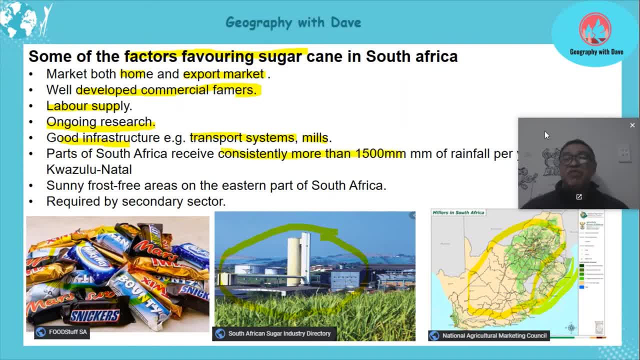 south africa receive consistently more than 500 millimeters of rainfall a year. example more along the coastal region, and maybe i should write coast. yeah, i must do some practice also. okay, and i'm gonna put an a here. all right in terms of my coast, right? i hope you're enjoying. 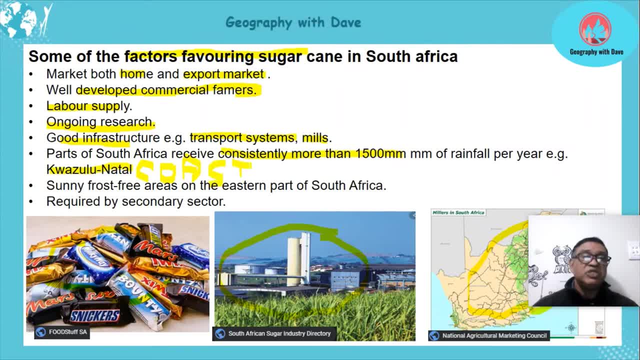 my writing. okay, the coastal regions receive a lot of rainfall. okay, and sunny, frost free areas along the eastern part of south africa, all right. durban does not have frost and i wonder if they get frost one day. they make frost men, i'm sure. okay, but they don't get frost, which is 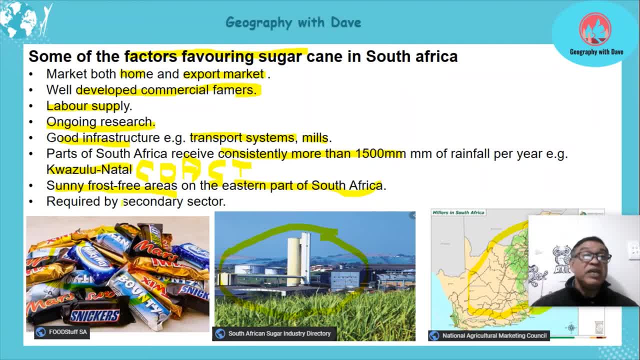 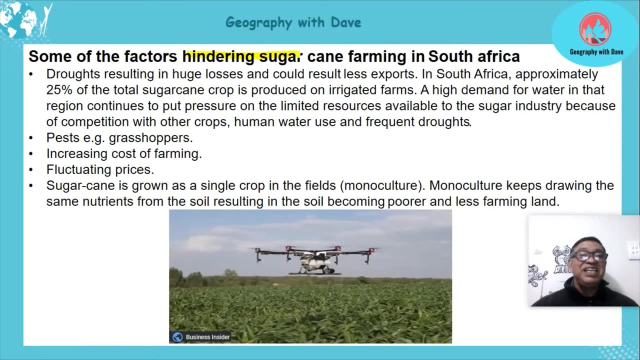 soon suitable for uh sugar cane production and, of course, it's required by the secondary sector, as shown by these chocolates. all right, let me switch this quickly before these chocolates torture me further. okay, some factors hindering. okay, droughts, can you see it? all right, huge factor. 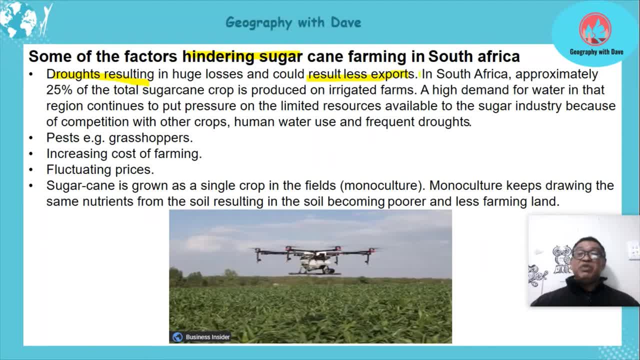 and it results in less exports. because then we're using here i'm going to talk about this- approximately 20, 15 percent of sugar cane is produced from irrigated farms. that's 25% recovered, that's four and one half. first of all, right, just. 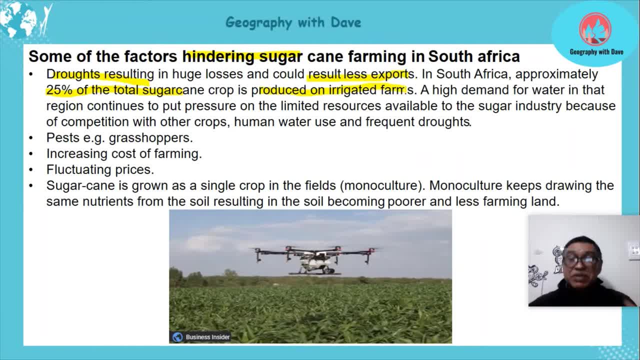 to illustrate some other factors here in this smaller problem. i just wanted to. i was looking at min instructions about artificial 사랑 and the ads say about 25 percent sugarcane being composed, while some series in the region you can see down here is location 25 percent� 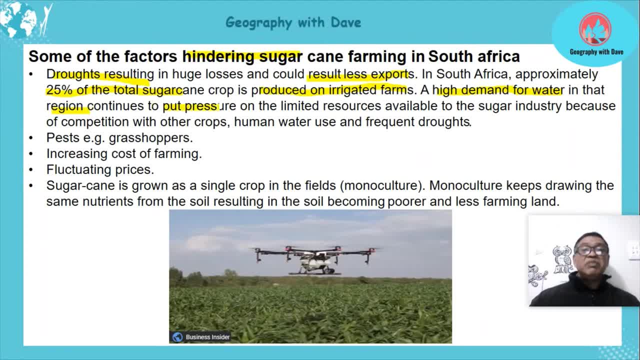 brachts from irrigated farms. all right, they don't have the nature. farms are irrigated by humans, you understand. so, 25 percent of the total, which is a quarter. okay, so therefore it's put pressure on limited resources available. okay, because of competition with other crops, other. 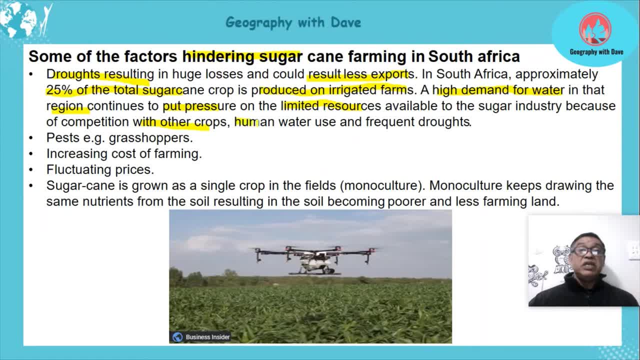 crops also need water, human water use and, of course, the frequent droughts. so we do need water supply, you understand, and sometimes the droughts make it worse when, even if it's stored water during droughts, you find the levels decrease because no water has been supplied into those. 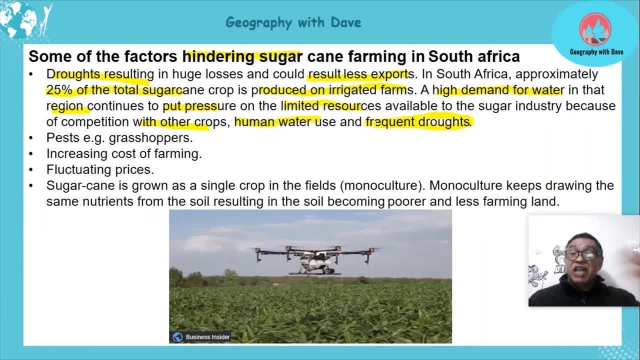 storage dams, etc. okay, and of course, the other consumption still continues. so it's a huge thing. droughts and, of course, uh, the reliance on water, 25 on irrigated uh, farms, etc. okay, piss, okay, like your grasshoppers, create havoc on these sugarcane farms and that is why you notice this. 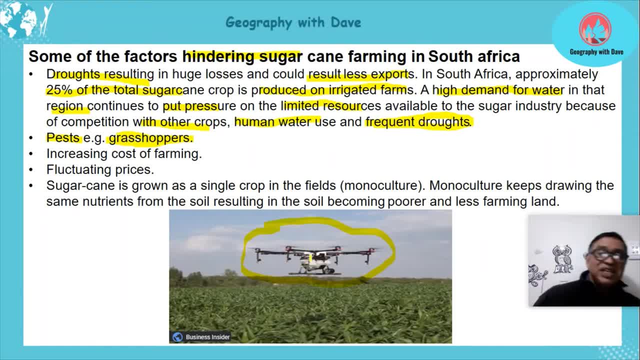 they're actually using drone now. drones now like this, all right, to actually spray the crops so it can keep away the insects, etc. quite interesting. of course, the increased cost of farming, which is another thing that all three have the same fluctuating prices, make it a problem up, down, up down all the time how much to invest in it. and you invest a lot. 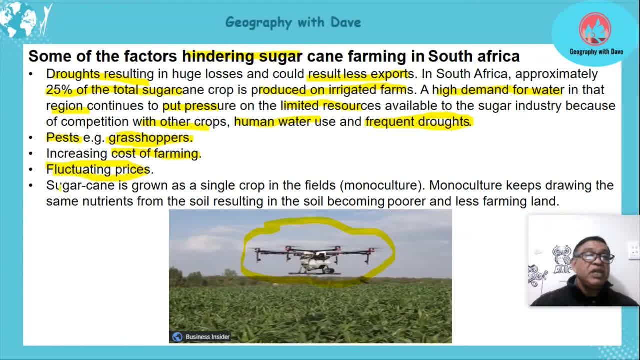 something, the price goes down. problem again. yeah, all right, sugarcane is grown as a single crop, okay. that's why we talk about monoculture, and each time you're drawing out the same nutrients by planting the same crop right from the soil- okay, and it could result in the soil becoming poorer. 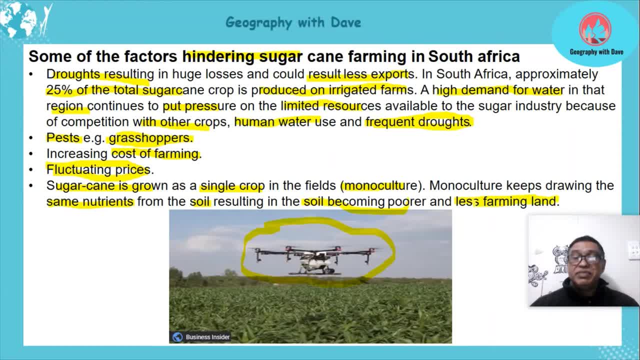 and less farming land, okay. in order to buy more land is always a problem. look, many of the commercial farmers will take steps to ensure that they put the nutrients back, but someday it's still a challenge which hinders farming as such. in terms of single crop farming, monoculture, okay. 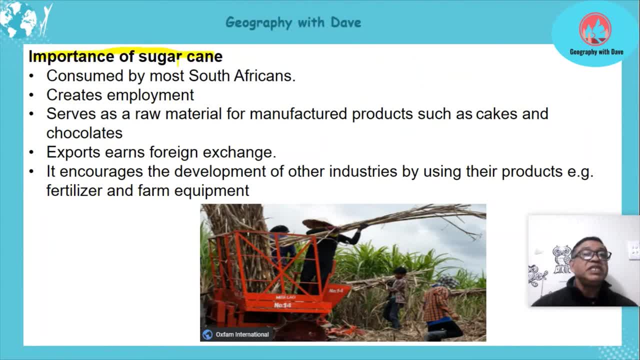 right importance of sugarcane. it's consumed by most south africans, maybe not so much of the diabetics, etc. who may not use the full thing from the sugar itself. they use alternatives. but it's consumed by most. but even those diabetics, i promise you, when they see those chocolates and 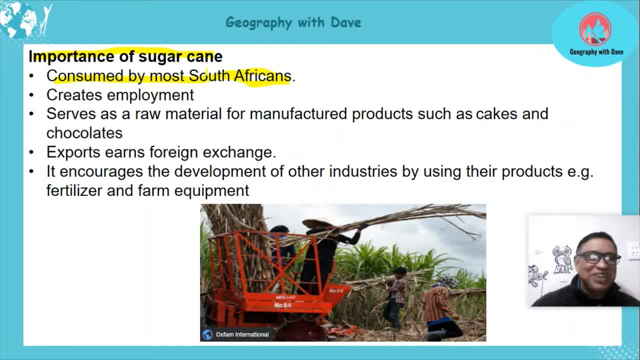 no one is watching. they're eating, so they're taking in sugar. right, it creates employment, as we said, in directly in the farming sector: secondary sector to make those chocolates, tertiary sector to actually sell the chocolates. whatever it's happening, it serves as a raw material again here. okay, like the other two products, but the different examples, like cakes, 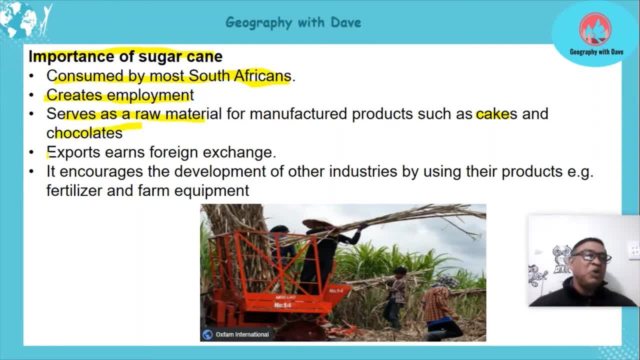 and chocolates need the sugar, and you know, i don't need to even explain this. it earns foreign exchange, a huge amount of foreign exchange. all right, okay, that money coming in. it also encourages development. okay, example for further of other industries, rather example: fertilizer and farm equipment. all these things supplied, all right. 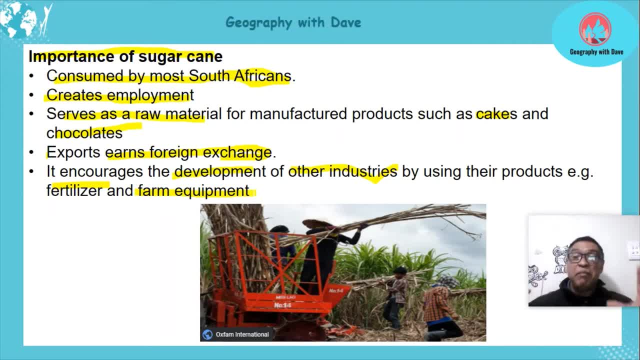 and therefore the production there and therefore these companies. as sugar improve increases, more of these companies are coming out. so all three products play a huge part in the south african economy. for balance of trade, to create a positive balance of trade, etc. or to try to move towards a positive- 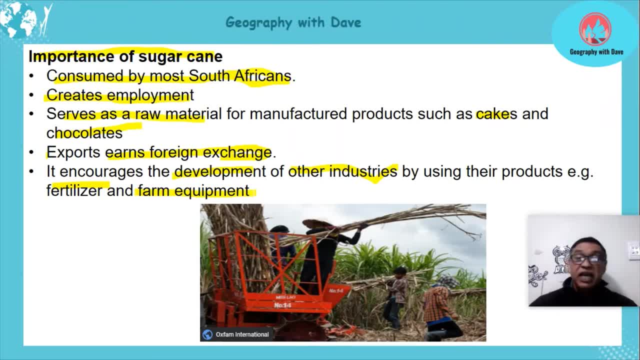 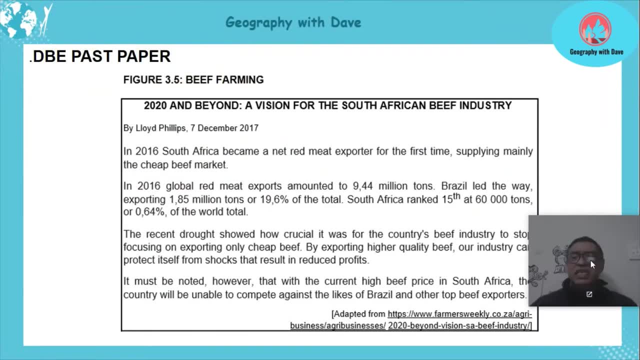 balance of trade, okay, plays a big part. all right, and that is why they are so, so, so important. okay, let's look at a db e pass paper learners, because we need to apply it. and that's always our style. we don't just get impressed by those chocolates and the piece of steak and the beef. 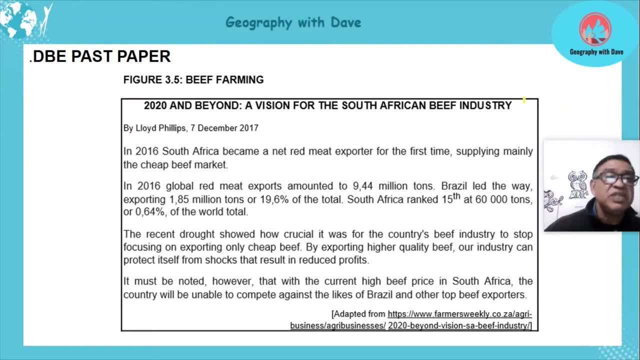 farming we need to apply in order to prepare for exams. so let's read this, of course again. our little heading all right, figure 3.5 is beef farming- gives us direction. already things through to our head about beef farming: right in 2016, south africa became a net red meat exporter- good news for south africa. for the first time, 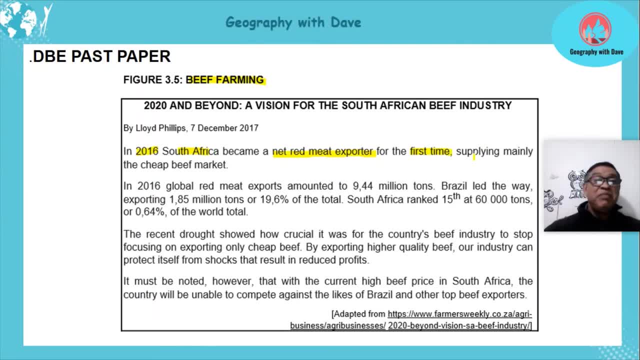 okay, can you see how much beef we eat here, supplying mainly cheap beef market? okay, like in 2016, the global red meat exports amounted to 9.4 million tons. brazil led the way with 1.8 million tons. so what has happened here? 9.4 million tons. 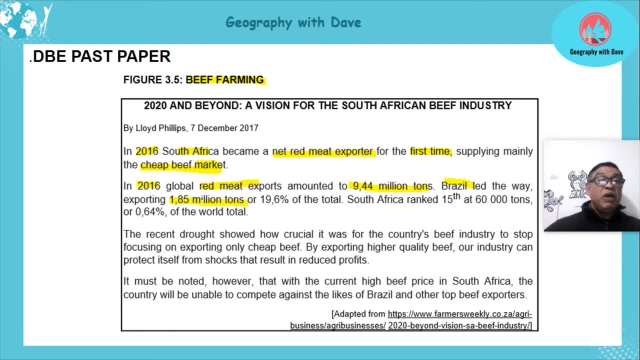 was the overall exports for the world, with brazil being 1.8 million tons. so they're the most, or 19.6, of the total. south africa ranked 15th with 60 000 tons. not bad 15th, all right, with 0.5 million tons in the world was the result of the standard at that time. 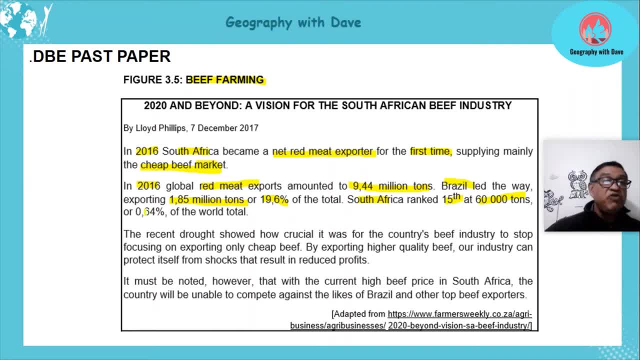 from the 1.8 million first to 19 ponto, determin todos in Bre Administração ca chegar aqui로 a~. Production price was all right, was 0.4 percent of the world. recent drought not nice, okay, uh, in the country showed. 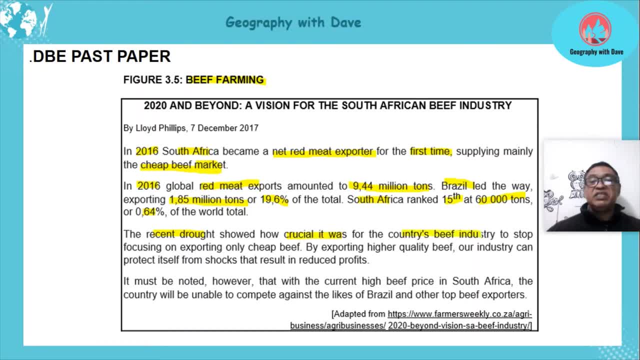 how crucial it was for the beef industry- the country's beef industry, all right- to stop exporting okay, and to stop focusing on exporting only chief beef. by exporting higher quality beef, our industry can protect itself from shocks that result in reduced tariffs. so what is saying this? because it's cheap, you're not getting so much money in. we should be exporting more. 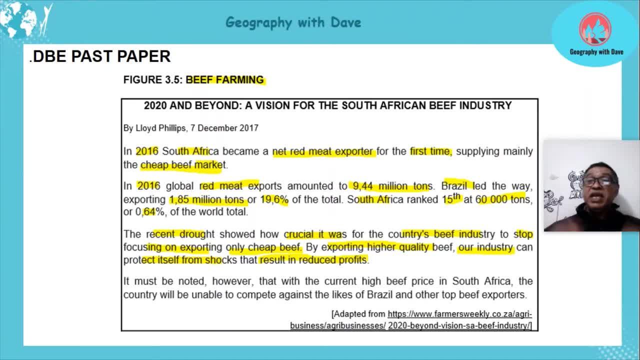 high quality beef at better prices. so more money is coming in and when these tragedies happen, like droughts, we have more funding available. it must be noted, however, that the current high beef price in brazil will be unable to compete against the likes of brazil all right and other top. 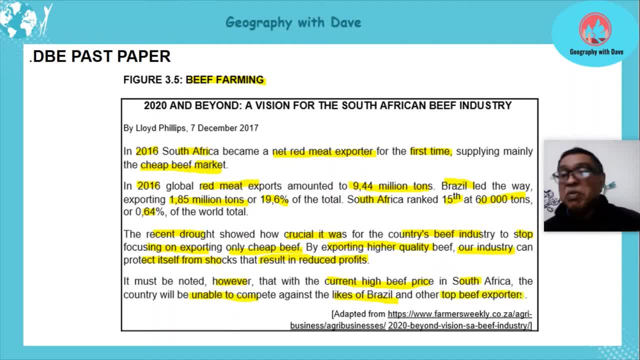 exporters because of the high price. brazil can be the bosses. they can play with their prices and each time we want to sell our beef they can reduce the price. you understand? so we can't really. we find it so difficult to compete with them. okay, so we went through the article and one thing again. 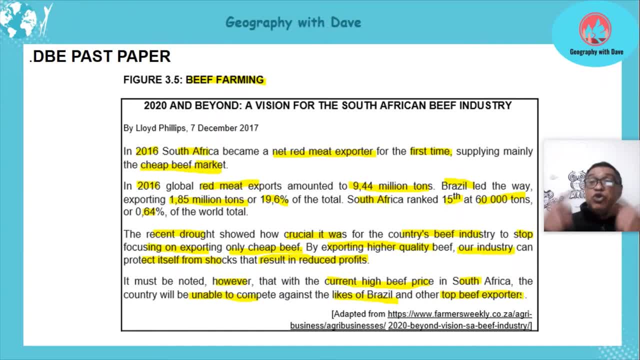 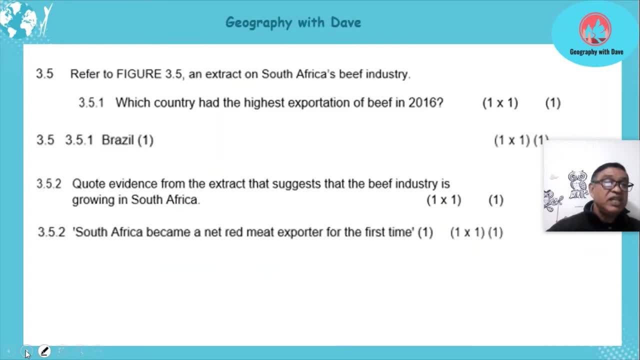 you most probably will find something from the article that will be useful. that is what the examiners do. remember that, okay, in all your sections. so let's look at it here. first one: which country are the highest exportation of beef in 2016.. can you see? that was part of the article. 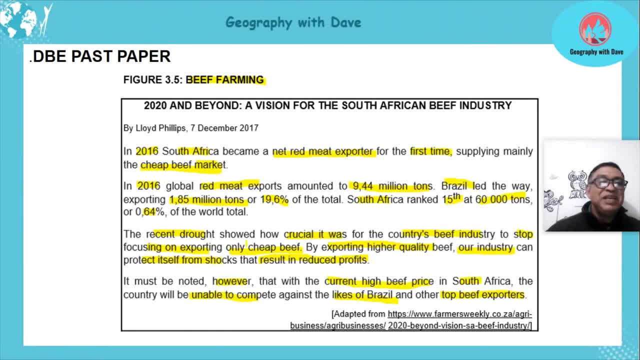 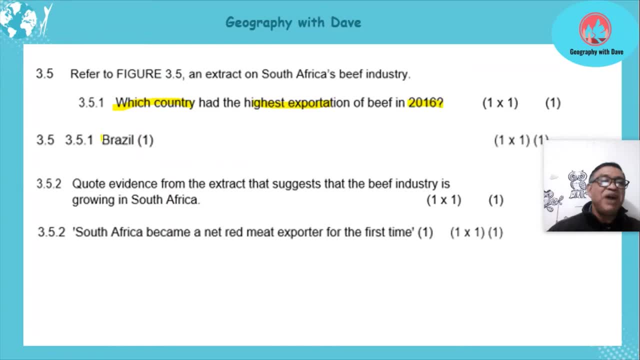 it was written there, lannis, can you see that it said a brazil, okay, led the way. so we got our answer there. it's good, eh, answers marks for nothing. brazil quote evidence from the extract that that the beef industry is growing in south africa. all right, why it can? we can only export if we have. 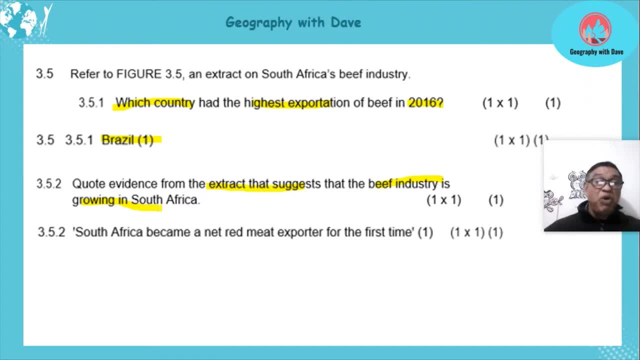 enough in the country and when south africa started exporting in 2016, meant that our beef industry grew, that we supplied the country and we was able to- uh, actually export. so the phrase there was south africa became the net red meat export for the first time, taken directly from the article. okay, learners, all right, let's go on. 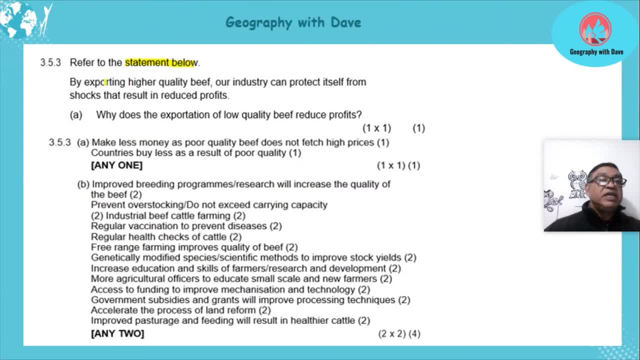 refer to the statement below. all right, by exporting higher quality beef, our industry can protect itself from shocks that result in reduced profits. okay, that's the first one. okay, now a what does exportation of low quality beef? uh, why does? sorry, why does the exportation of low quality beef? 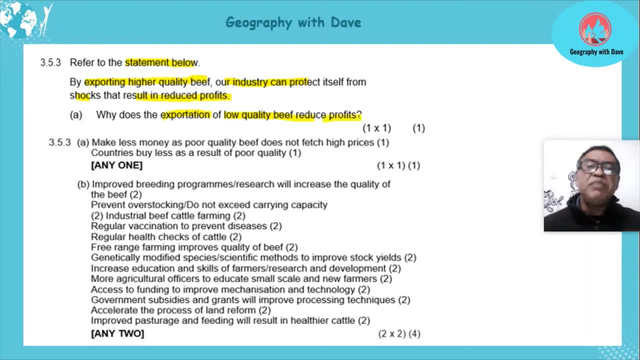 reduce profits. now what i'm picking up on this and that is why i put this in: okay, uh, it's brought in. exportation of high quality, exploitation of low quality, all right, and these words that come out, you say, oh god, i didn't cover this, but you have, and sometimes you have to think out of the box all. 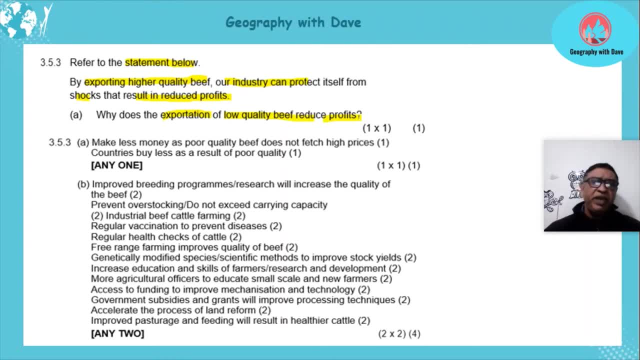 right, and some of these questions are not difficult. it comes from there, all right. low quality beef sold at low prices. high quality beef sold at high prices. so look at the wording also, learners, in order to get your answer. so let's look at the answer. makes less money. 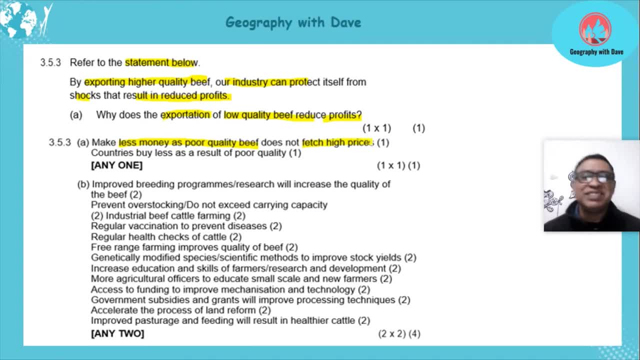 as poor quality beef does not fetch high prices. can you see? it's logical, so don't get shocked. you know, sometimes we learned it in parent fashion. as we say, we just learn our notes. therefore, we can't read into the question on what it's saying and you'll be able to answer it. okay. so countries buy. 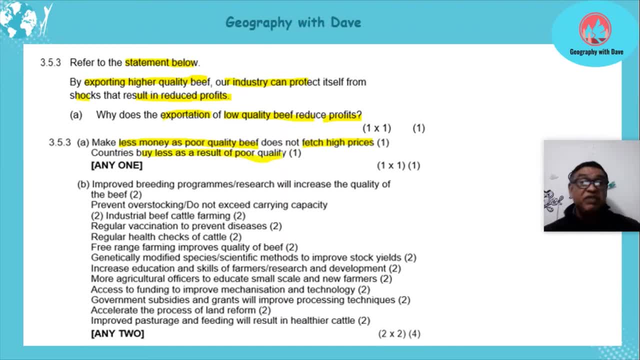 less as a result of the poor quality one of them, it brings in less money and, on the other hand, if it's poor qualities, country doesn't want to buy. they want good quality for their people, right, that's one of them. okay, then, b? uh we talk about here and i don't have the 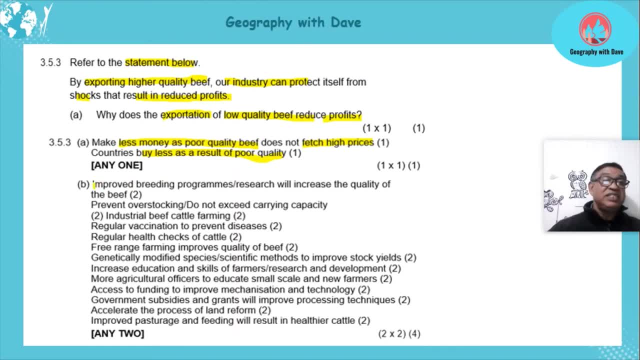 question here. i must apologize for that. it says: improve breathing programs and research. uh. prevent overstocking. all right of. does not exceed the carrying capacity. these are measures that can be introduced. all right in terms of uh protecting or improving the beef industry. so my apologies here, all right for not having the 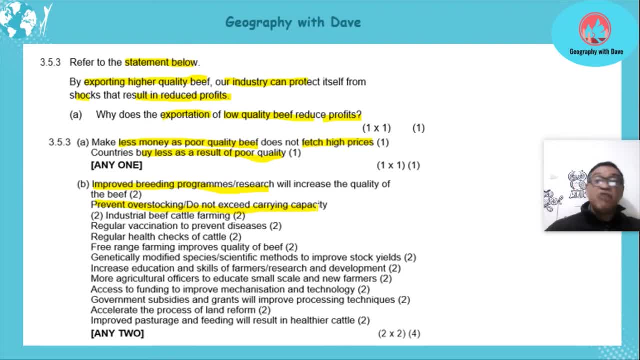 question. i do apologize, learners, but ways of improving the beef industry, can you see it? and, of course, reducing uh things like uh debt rate, etc. okay, can you see industrial beef cattle farming? okay, uh, regulation of vaccinations to prevent diseases: can you see it? all important regular health checks for cattle. besides you having a health check, they must have a health check. 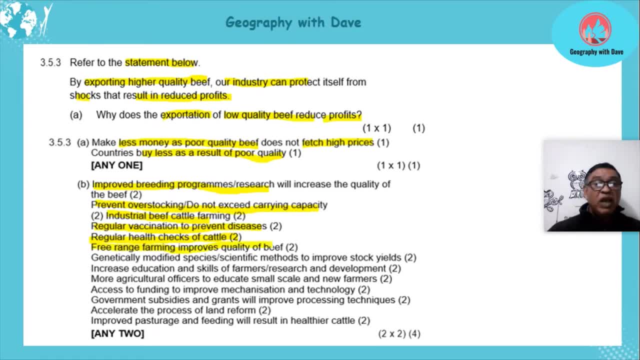 all right. free range farming improves quality of beef means free range. allow them to eat on the natural vegetation, can you see? so my apologies for the question learners, but ways of improving beef farming would probably be the question down here. all right, so we look at others genetically. 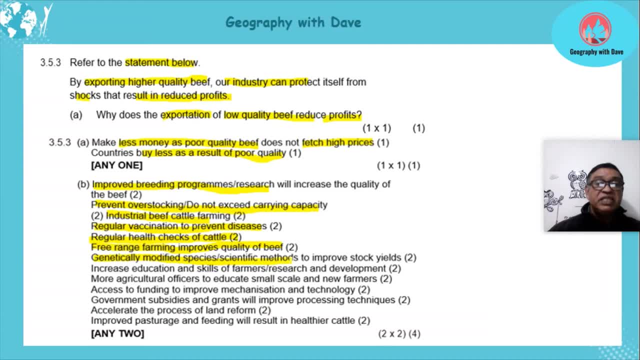 modified species and scientific methods to improve stock yields. okay, by having genetically modified, you find cattle become stronger. all right. okay, and the yields are bigger, bigger cattle, etc. all right, because it's genetically modified. increase education and skills of farmers. okay for food and development. so when you teach them more skills, they'll be able. 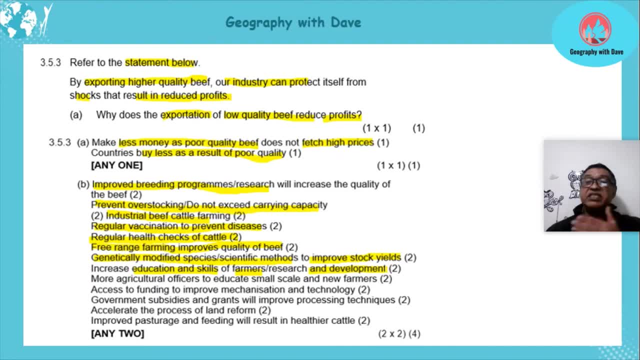 to implement better methods on the farm. less capital dying, better quality cattle- okay. more agricultural offices to educate small scale farmers: okay. who are farming on a smaller scale for commercial basis: send advisors like agricultural officers, okay, that will go there and will advise them. listen, this is what you can do to improve your production. okay. excess funding: 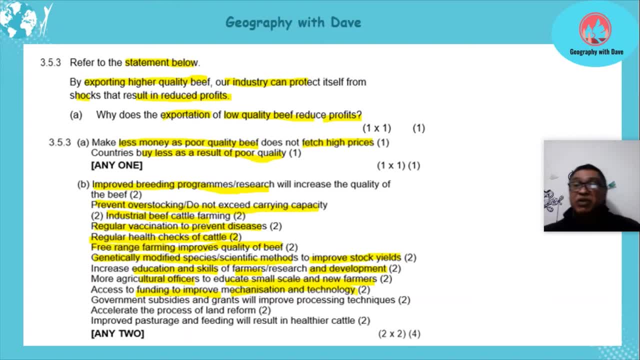 to improve mechanization and technology. okay, funding forward that we have more technology being introduced, finding new methods. you understand, so it improves it. more technology, better quality cattle, better survival of cattle- okay, milking of cattle, etc. all these things will be there. government subsidies and grants will improve. 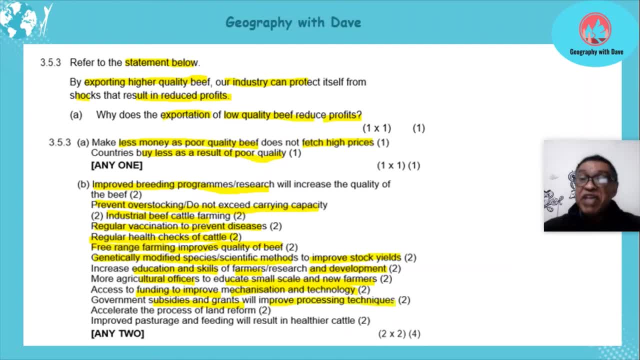 processing techniques. so more of that, all right, processing techniques, processing off of cattle, etc. into various, various other products. if you have more of this it will help accelerate process of land reform. okay, of course, if the focus giving back land. you know you've done in settlement geography land. 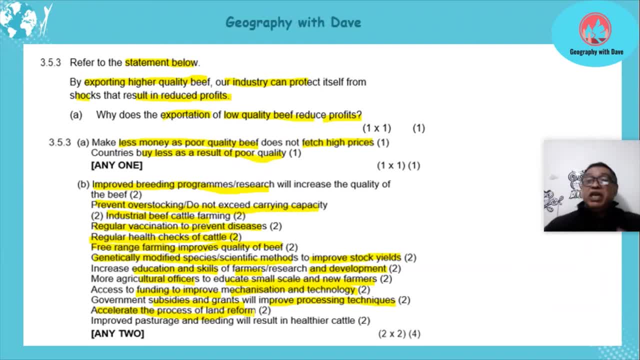 restitution, land redistribution, etc. okay, give it, but of course it needs to be intelligently done. okay, when giving back land to be used for farming, we need to help farmers financially educate them in regarding the skills so that more can come in, not just pass over the land. okay, it's very. 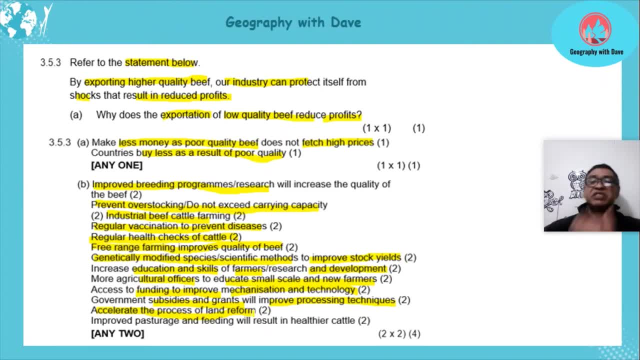 very important. people in south africa have intelligent minds and if we educate them about the importance of of, of farming, etc. you understand of beef farming- and we get them involved, we provide the funding. we can go forward and increase the production. okay, improved pasturage and feeding. 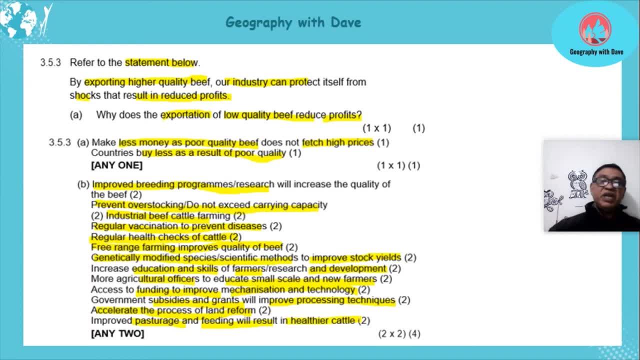 will result in healthier cattle. okay, so learners, please know. the question was improving beef farming. okay, i don't have the question in front of me, but we're going to assume it. how could we improve beef farming in the country? and once again, my apologies for not writing. i think it was those steaks and 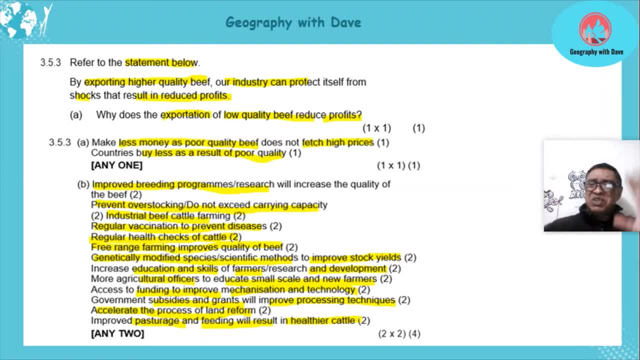 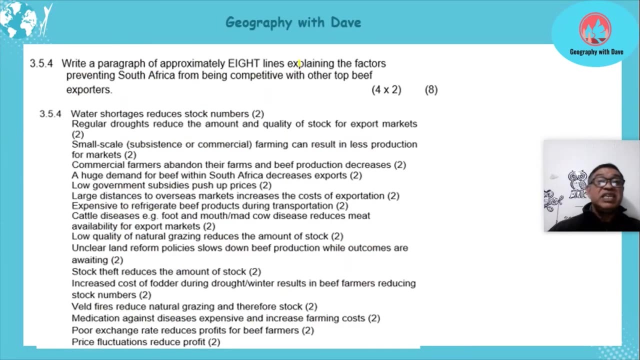 the chocolates that took my mind off it when i was fitting those in. all right, it made me too hungry. therefore, i left the question out. okay, my apologies. okay, right. then the next question: write a paragraph of approximately eight lines, and once again i'm saying: all right, it's about eight lines, it can be more or less, depending on. 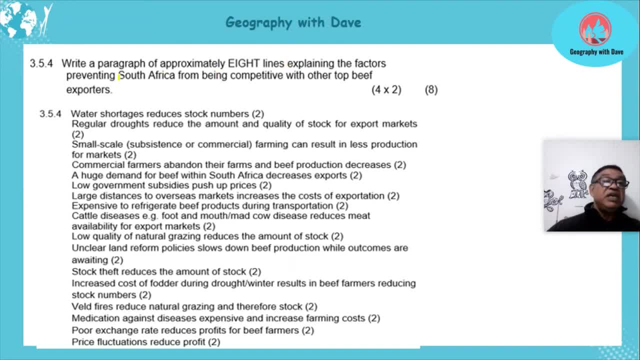 the size of your writing. some of your writing is so big you can use remote sensing and get identified from outer space there. okay, so you'll use more lines. all right, eight lines explaining 입. so your seven did not look at the word preventing images when factors favoring. all right. 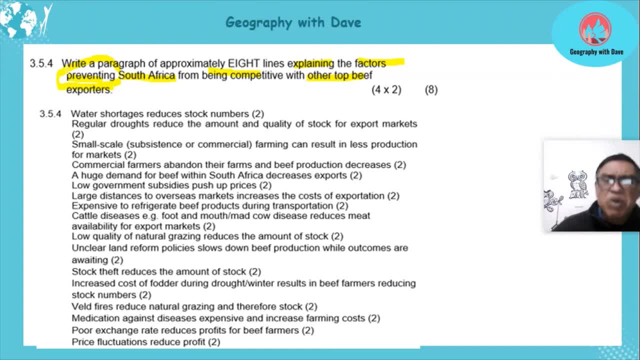 it's preventing- watch the words, so important, you know your work, you understand, but because you have not actually read properly, you can have a problem. so it's preventing, stopping us all right from becoming more competitive, stopping us from competing with the top beef exporters like Brazil. what other? 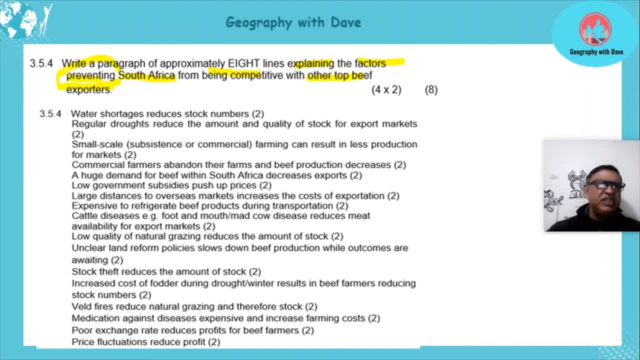 factors. we gave it straight from your modes factors, endearing, etc. all right, look at this. water shortages, didn't we deal with? droughts reduces stock numbers, okay. regular droughts reduce the amount and quality of stock for exports. can you see it? it's phrased in different ways, which means we can. 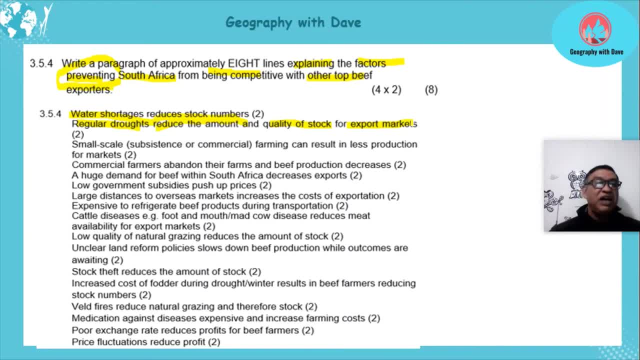 take droughts and explain it in different ways. all right, so gate, what is it Friday hawks? all right prices, like僕 ways we'll get the marks. small scale subsistence and commercial farmers can result in less production, so we need to encourage them to produce more. so examiners have been nice. can you see they? 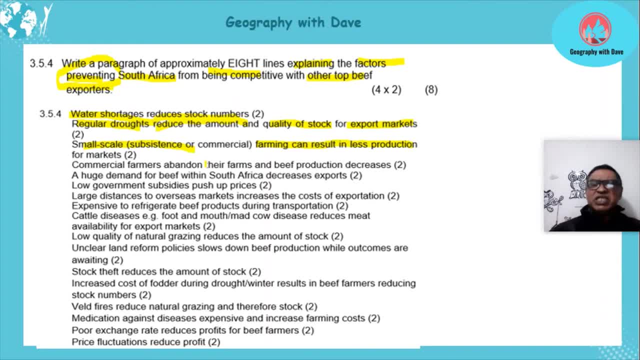 give you so many alternatives. okay, so you sit as long as you put in a full thing. you understand, you explained it fully. you don't just write water shortages and that's it. no, it says: explain: water shortages reduce stock numbers. regular droughts reduce the amount of and quality of. 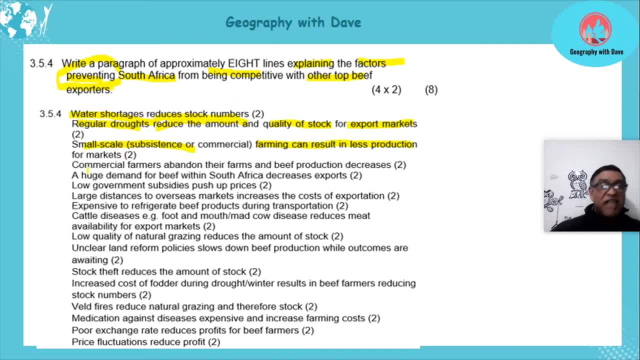 stock for exports. can you see? you have to explain it fully, learners. that is the important thing. commercial farmers abandon their farms and beef production decreases could be for various reasons: drought or their money loss, etc. huge demand for beef within south africa decreases exports. can you see what we're doing, learners? we are taking. 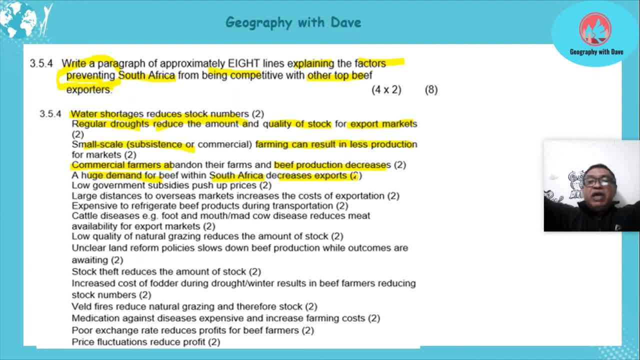 those points. all right, that we've learned, okay, that the consumption in the country is high and we're applying it to our answer. can you see we just tweaked it a bit and made it correct for answer and explained it fully. no government subsidies push up prices. all right, because 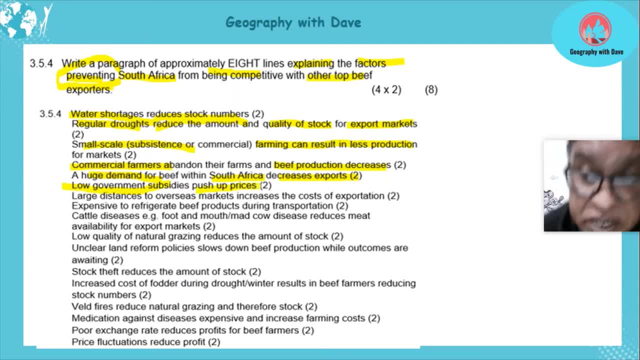 we don't subsidize in our country. that's another point. okay, an external point down here, but you will have enough from your notes to write. okay, we can see there's a whole lot of points here. all right, so you have enough. if it's four points, you have four points already. 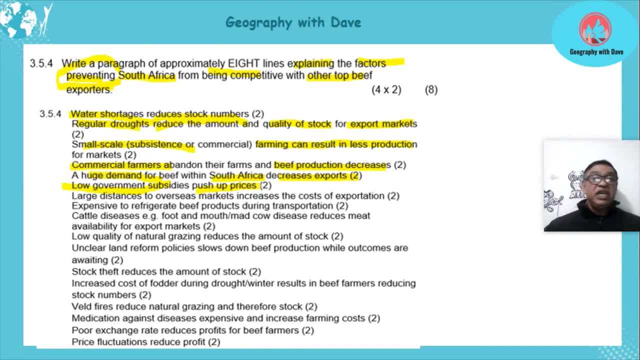 but the examiner has to give all the alternatives. you understand, because people may have read something in a paper. you may have read something in the paper right: large distance to overseas markets increase costs of exploitation. can you see how we think along the way? could have read that: okay, so expensive to refrigerate beef products during transportation. it is expensive. 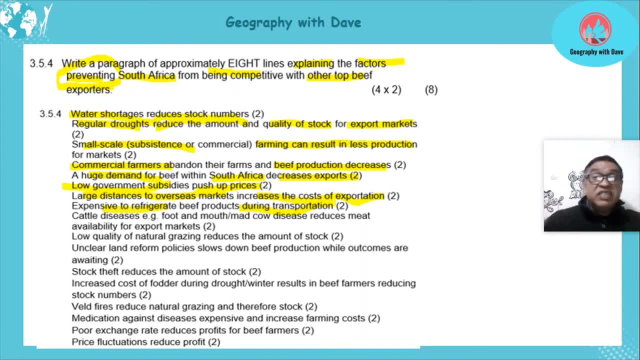 you pay a lot of money, all right, because these things have to be frozen, otherwise it's not going to be nice when it gets there. cattle diseases: can you see? foot and mouth. mad cow disease: reduces meat for exports. can you see? it's all in the notes. low quality natural grazing reduces the amount. 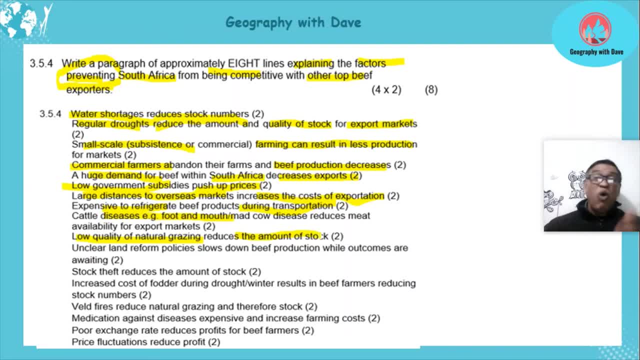 of stock. an additional point. all right now. you don't have to know all the points. learners remember, if you know four to five points, you are fine. no more than four points, because it's out of the most points you can get is four. in a paragraph question which is out of eight, you have to give four points. so I would say: if you know five, proper. 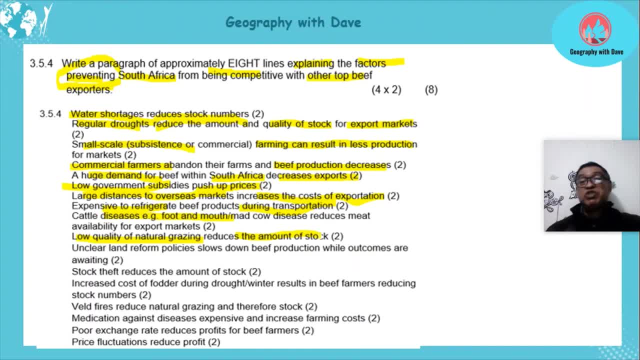 points. you understand it must be. if they could ask you: economic, social, need, to know five of each. but sometimes it's general like this: five points and you got your stuff, you don't have to learn 20 points. okay, unclear land reform policies: okay, well, maybe land is just given. okay, slows down. 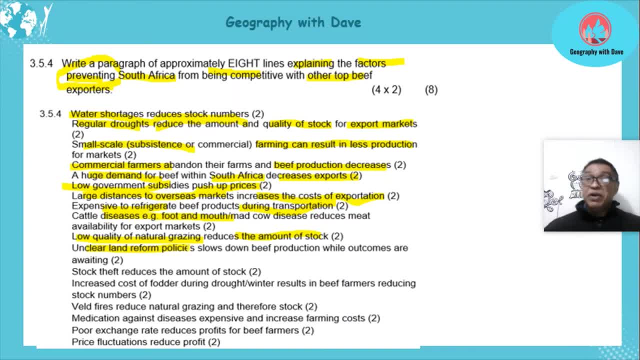 our beef production. okay, of course land needs to be given back. all right. there's nothing wrong with land reform policies. as you learn, people have lost their land over the years, you understand. but it has to be done in a proper way that would encourage activity. that will promote economic activity in. 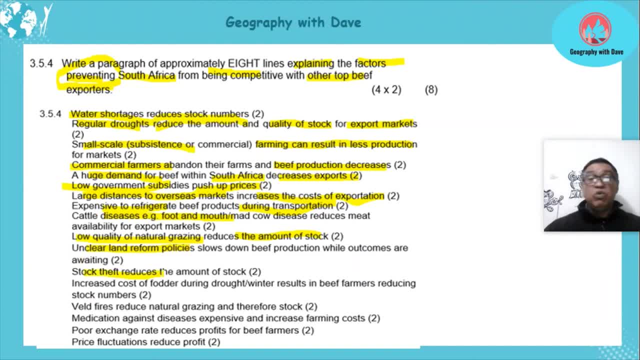 our country. stock theft reduces the amount of stock which happens in our country. increased cost of father, remember we said increased cost of the farmer. we brought in here the fodder. maybe the market becomes more expensive. felt fires: okay, remember you've done all those things before, eh. regarding uh bug wins, Etc. firefires are common in our country, okay, which can damage uh uh natural. 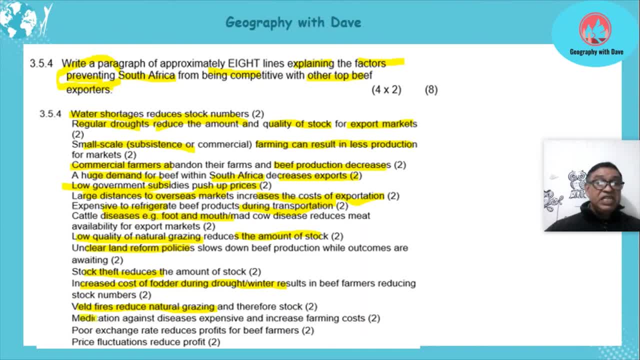 grazing field and even kill animals. medication against the disease is expensive, which improves, increases the farm. the costs, all right. poor exchange rates reduces profits for beef farmers and depending where they are selling, all right. and sometimes these poor exchange rates where the value is lower means they're getting less money into the country when it's 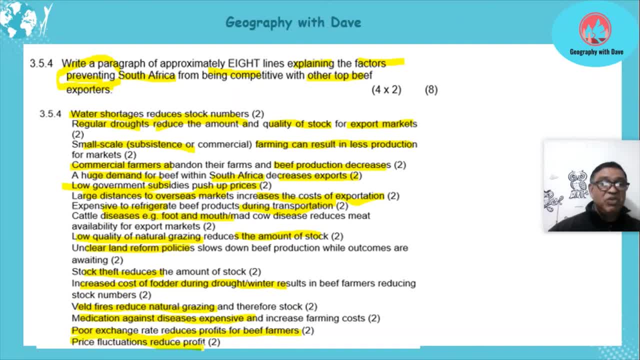 exchanged price fluctuations. can you see that also? so out of this price fluctuations- it's hard- reduces profit if the money goes, if the price goes down, less profit. can you see out of this whole list of all these factors, quite a few in your notes already. it means taking it, tweaking it a bit. I use the word tweaking I. 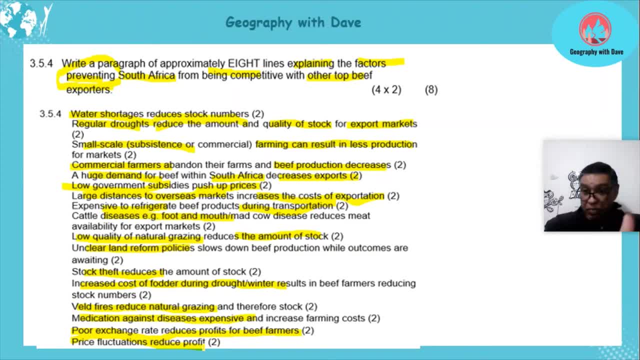 like that, tweaking it a bit and making it appropriate to what the question asks for. okay, so that's how you answer, let us- we've now done the main products in terms of our agriculture. I hope you enjoyed the lesson and I hope you liked looking at that piece of steak. 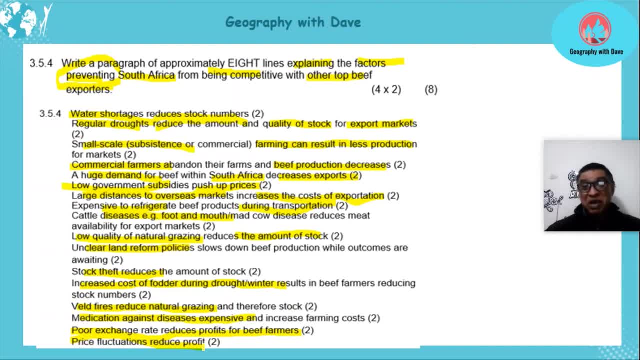 I know you will be at school at the moment watching this program. don't bunk school. make sure you finish. try and contact your parents after that, as you're going home, to make that steak for you, because I'm going to go now and have a piece of steak. whoa, I'm hungry, all right. that is all the best, goodbye.